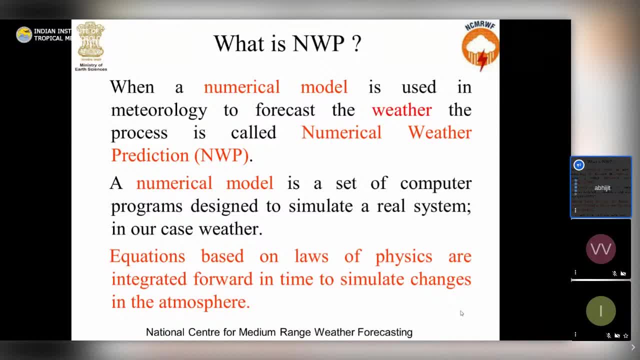 we call it as numerical weather prediction. It is a set of computer programs that are designed to simulate a real system like our weather, And the basic laws of physics are written in terms of differential equations, And those differential equations are integrated forward in time. 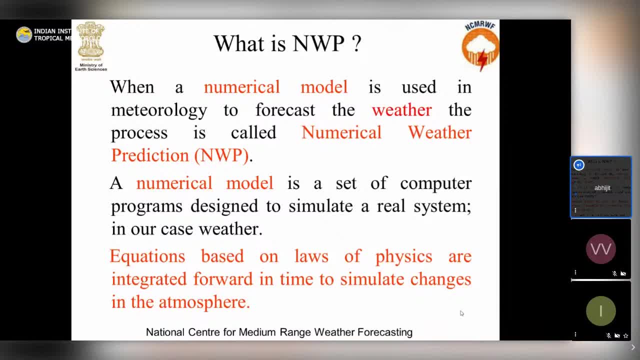 We call this solution of these equations And the method of solution of these equations are written in terms of computer programs. Those computer programs are run within a computer as if the future state of the atmosphere will evolve within the computer starting from a prescribed initial condition. 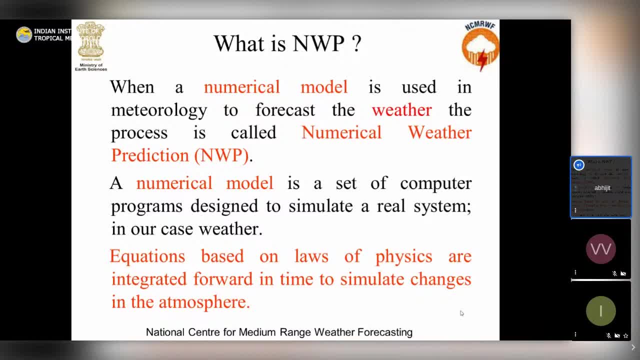 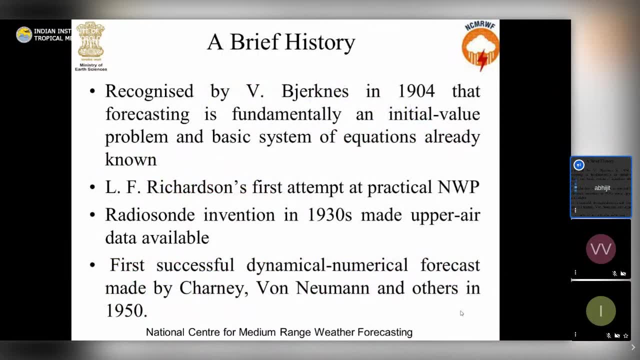 So this whole process we call it, is NWP, Or numerical weather prediction. This idea that this numerical weather prediction can be done by solving these equations representing the basic laws of physics starting from a prescribed initial condition was first recognized by V Barclays in 1904.. 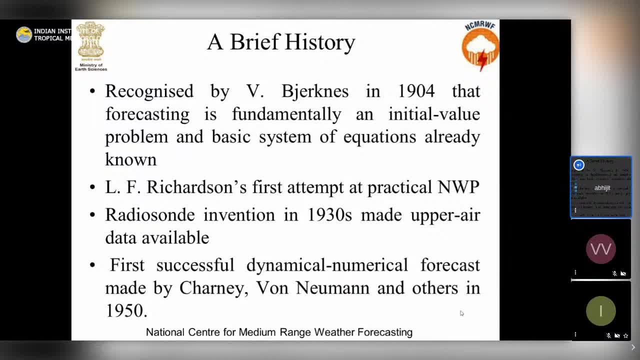 And in 1922 LF Richardson published his work of first attempt of NWP. But his attempt was a failure And he could predict within six hours time a pressure change of about 145 HPA, which was totally unrealistic. But he anticipated that maybe a huge number of about. 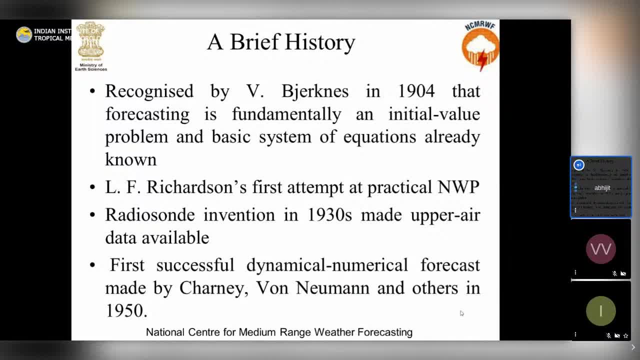 64,000 human computers. if we can put so, then they can predict the weather well in time and can give accurate forecasts. Then radio sondage was invented in 1930s. So with the invention of radio sondage the data from different levels of the atmosphere started coming. 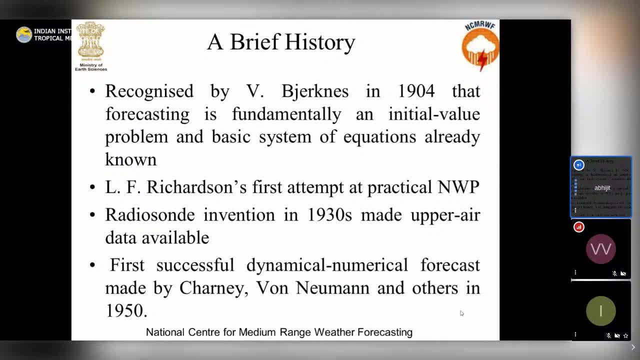 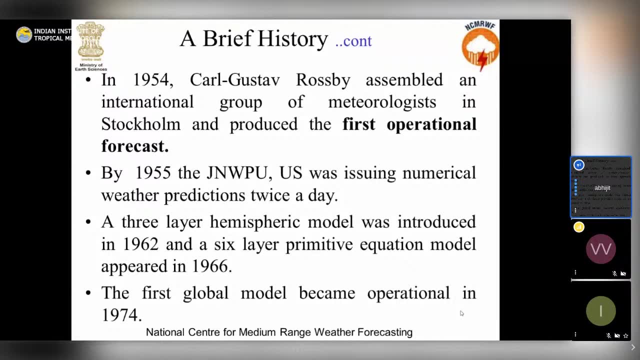 to the meteorologists, And then fast, successful dynamical numerical forecast was made possible by Charley von Neumann and others in 1950 with the help of ENIAC computer. In 1954, Rosby with his group of scientists produced the first operational forecast. 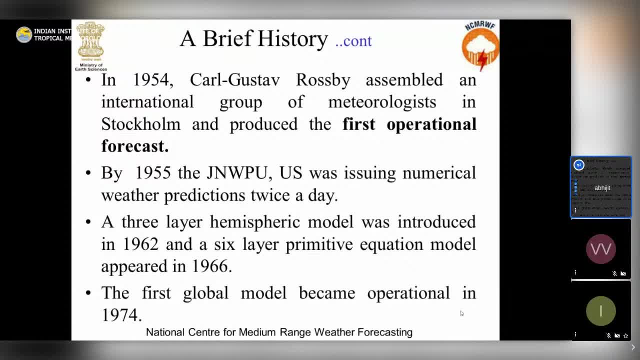 And in 1955 the joint numerical weather prediction unit of US, that is combination of US Air Force, US Navy and US Weather Bureau. So that was issuing numerical weather prediction twice a day And a three layer hemispherical model was introduced in 1962. 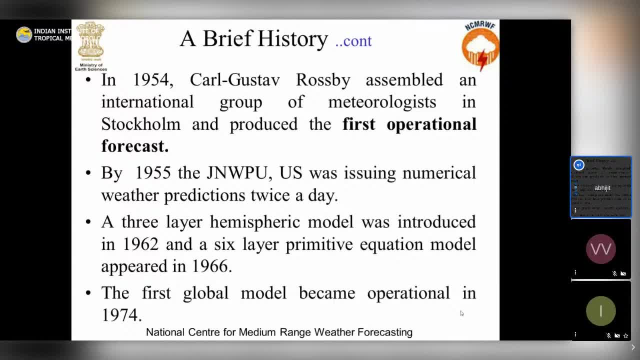 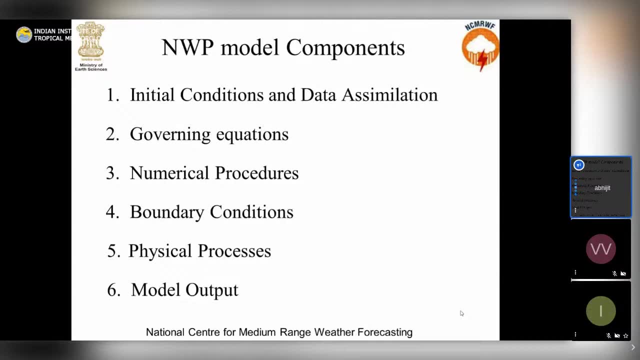 But the first global model. it became operational in 1974.. So this is the basics. This is the brief history of NWP. Now let us see that. what are different components of NWP? So, since we have to start from a prescribed initial condition, 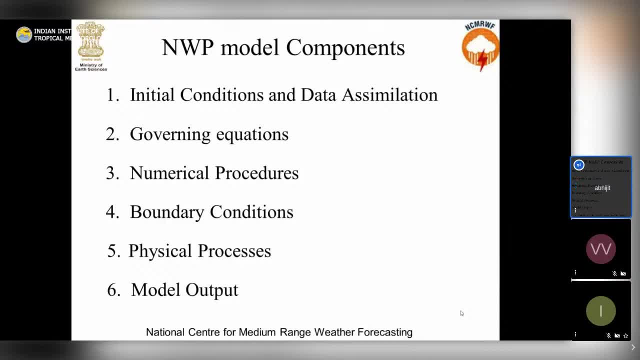 so first I will talk about initial conditions and how these initial conditions are prepared with the help of a method called data assimilation, And then I will discuss about what are the equations they use For these NWP And then what are the how we are solving these equations. 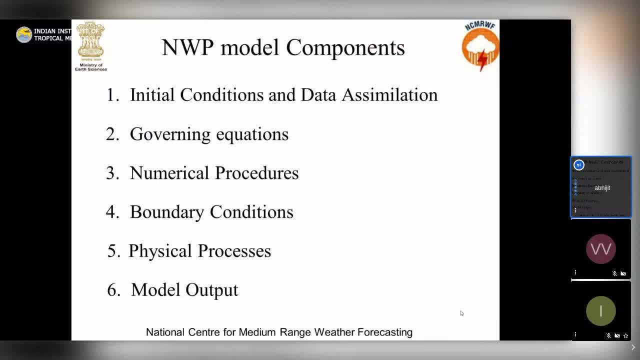 through numerical methods And we have to always prescribe the boundary conditions. So I will talk about boundary condition, Then the physical processes that appear through the source and change terms in these governing equations. How to handle those physical processes. that also I will discuss. 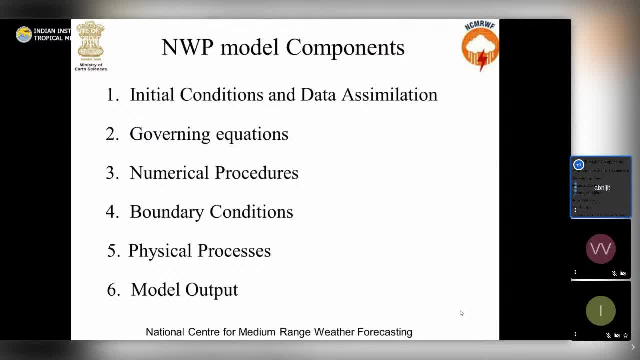 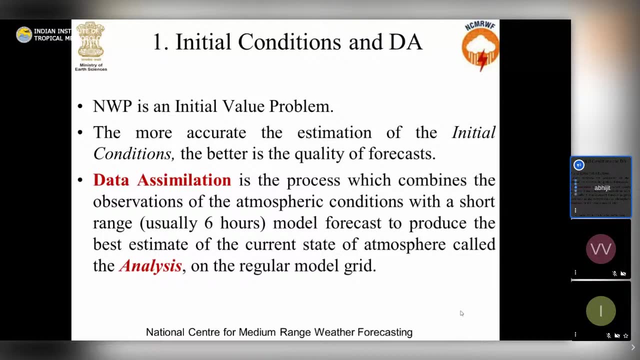 And finally, how we get the model output And how the uncertainty is associated with these model output, with these NWP different components that also I will discuss. I have already told that NWP is an initial value problem. The more accurate the initial condition, the more accurate will be the forecast. 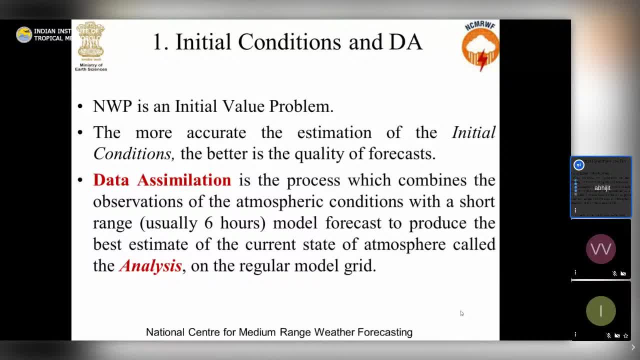 And data assimilation is a method which combines two informations- One is from observation, Another is from a short range weather forecast- to produce the best estimate of the current state of the atmosphere And that we call as analysis. So we prepare this analysis on a regular model grid. 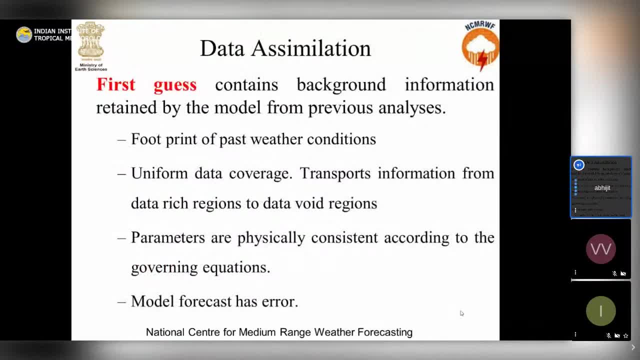 First, the first component is first guess. So that is the short range weather forecast that we use as the first information. We call it as first guess And it contains the background information which is retained by the model from previous, all the previous analysis. 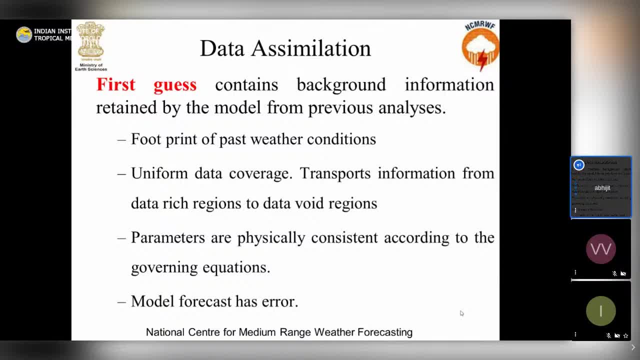 So we can tell: this first guess is the footprint of all the previous observations and all the previous analysis And since we are producing this first guess over the model grid, so that it is the data coverage is uniform, And all these previous observation, scattered observations, that information through model. 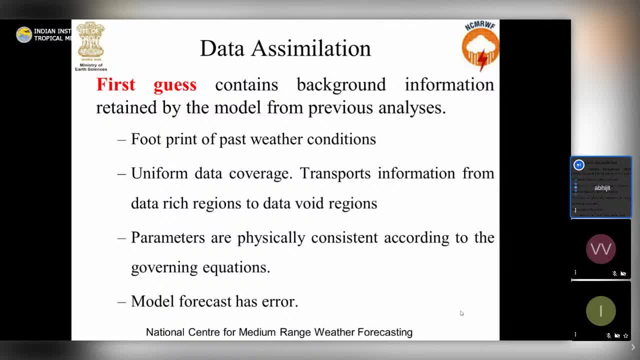 it goes from one grid point to another grid point, so it transforms the information from the data reach region to data void region And parameters are physically consistent according to the governing equations, But still it is a model forecast and the model forecast has some error. 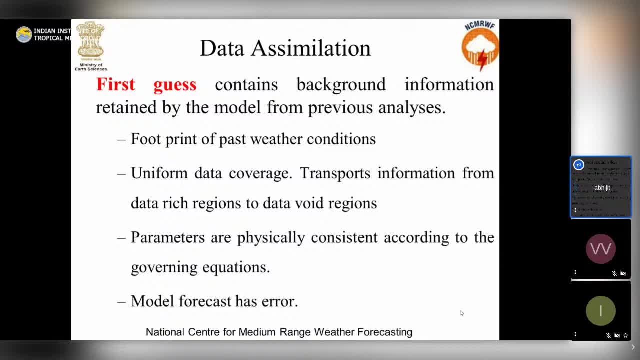 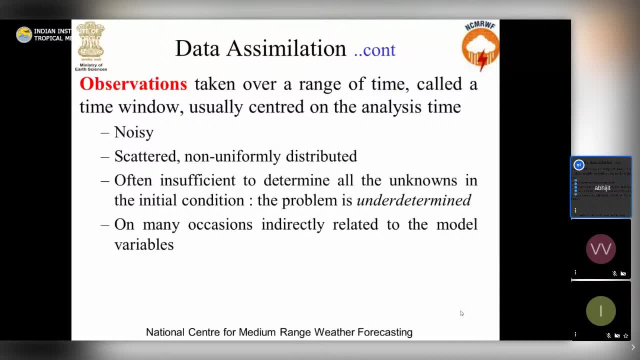 So first guess is erroneous. And second component is observation. Observation taken over a range of time. we call it is time window And the time window center is at the analysis time. But the observation is also noisy. Moreover, the observations are scattered Somewhere the observation density is very large. 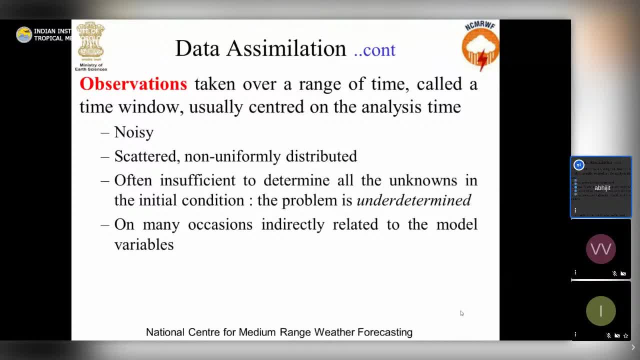 Somewhere the observation is sparse. That means it is non-uniformly distributed, And this observation is often insufficient, So it is insufficient to get the information throughout all the model grid points. So we can tell the problem is undetermined And on many occasions 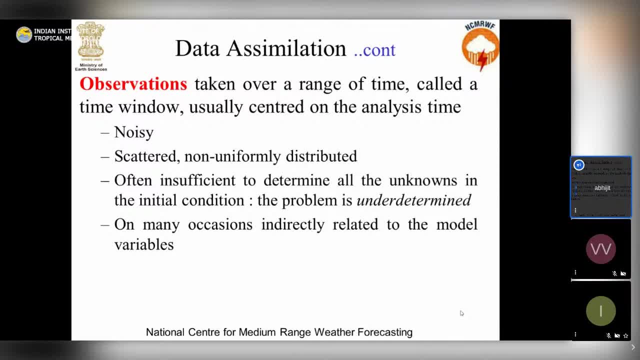 it is indirectly related to the model variables, Like satellite radiance, So this is not the model variable, Model variable. associated model variables are temperature and humidity. So we have to somehow convert this model variable, with the help of an observation operator, to the observation variable. 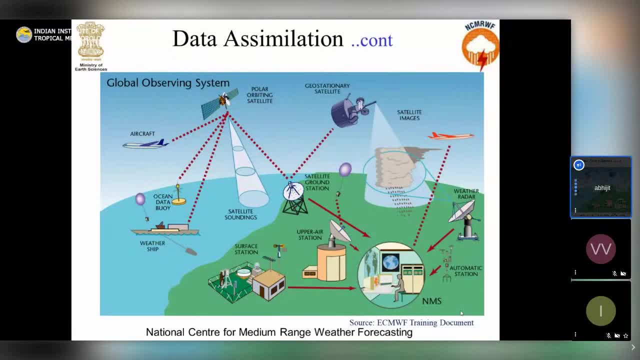 And these are the global observing systems. So we get the observation from different sources: through satellites, through radars, wind profilers, through seeds, GUI, the surface observatories. So from different sources we get the observations And these observations have different types of errors. 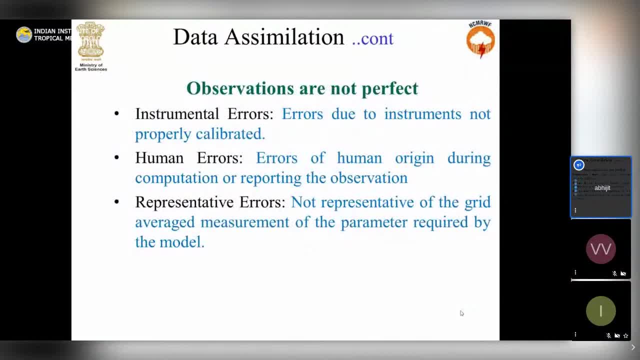 It has the instrumentation errors And these errors may be of human origin during computation or reporting the observation, And even if the observation is correct, but it may not give you the grid averaged value which the model is expecting. So, although that fault is not of the observation, 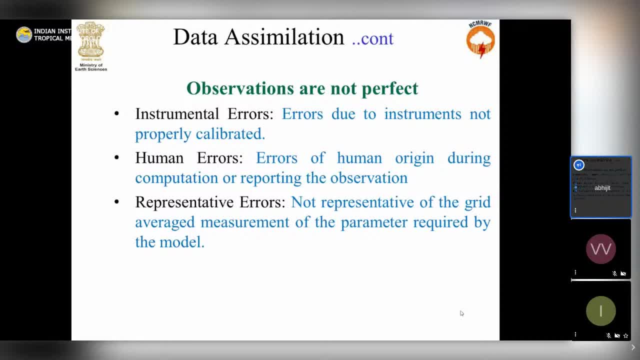 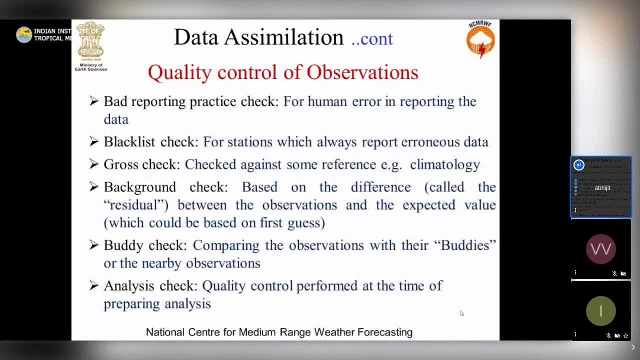 but the error is attributed to this observation as representative error. So first we have to do quality control of these observations. So there are different types of checks. One is bad reporting, practice check, So that takes care of human error in reporting the data. 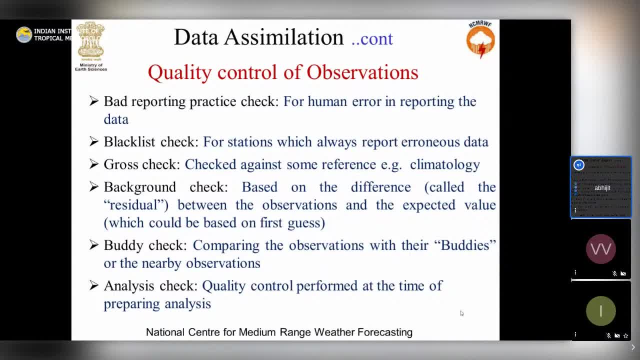 Some stations they always send the bad observations or erroneous data. So that goes through blacklist check And then the observation passes through gross check, which is checked with respect to some climatology, And then it passes through background check. So that means we compare how much it is different from the first guess. 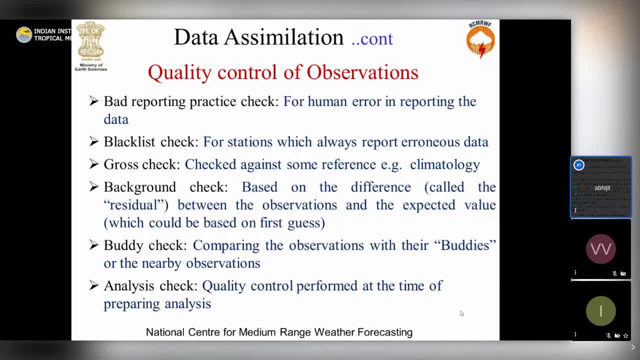 Whether it is enormously different from the first guess or it is consistent with this. whatever the differences usually we get with respect to the first guess Even it is even the difference if it is very large, so then it can pass through body check. 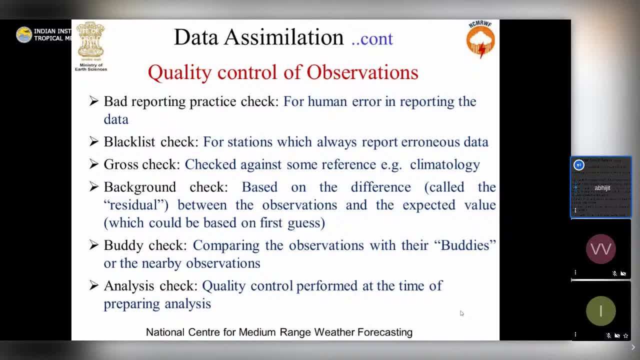 Body check means it will be compared with neighboring datasets And suppose all the checks becomes failure, then also the data is not totally rejected. So during the analysis procedure when the first guess gets updated, so those data are again checked that whether it can fit into the process of the assimilation. 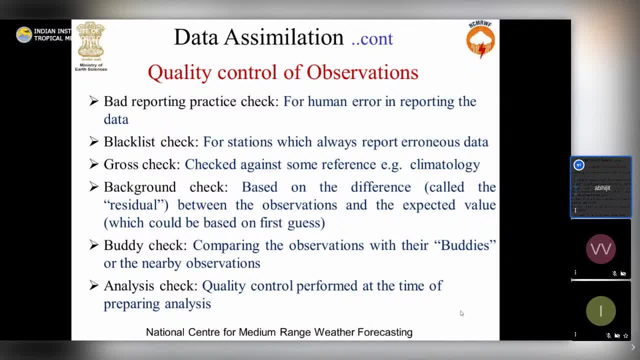 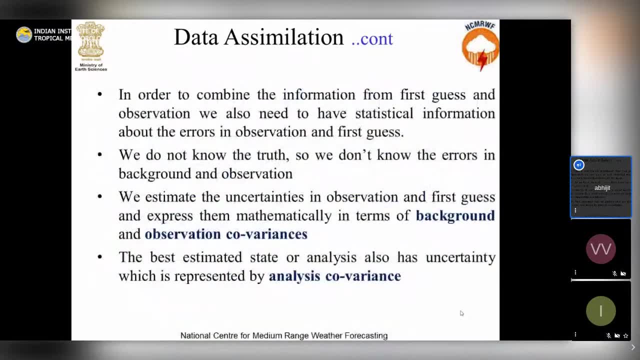 So through this quality control methods, we select the observations for the assimilation. So, but not only the first guess and observation these data, they are required for the whole process of data assimilation. We have to know some statistical information about the errors of those data. 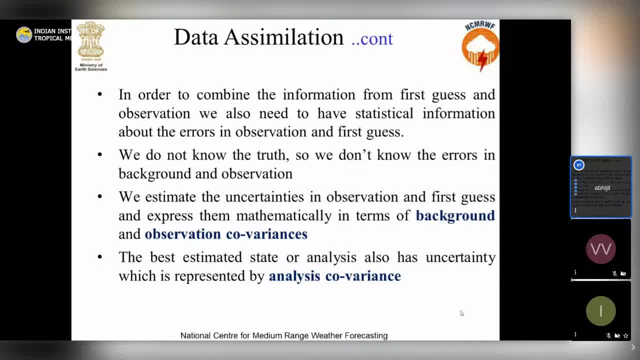 We do not know the truth So exactly, we don't know how much error is associated with every type of information, But we can estimate the uncertainties associated with these, both type of information, that is, observation and first guess, And we express these uncertainties as the background. 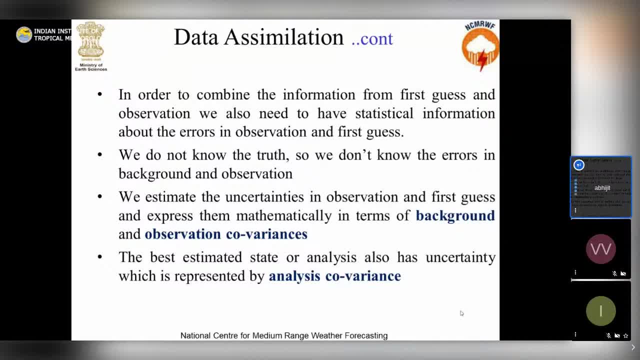 and observation covariances. This background and observation covariances, it gives the measure of the uncertainties and also it gives the relation between the uncertainties of different variables at different locations, The best estimated state of analysis, that is, that also has uncertainty and which we call analysis covariance. 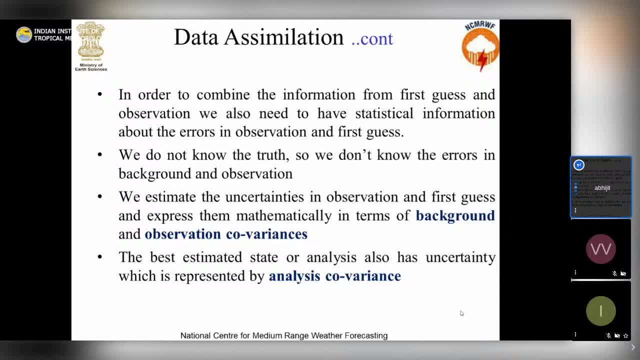 So we have uncertainty in first guess, we have uncertainty in observation and then from there we try to create best estimated state of the atmosphere. but it is not the true state of the atmosphere. And the best estimated state of the atmosphere has also uncertainty that we measure. 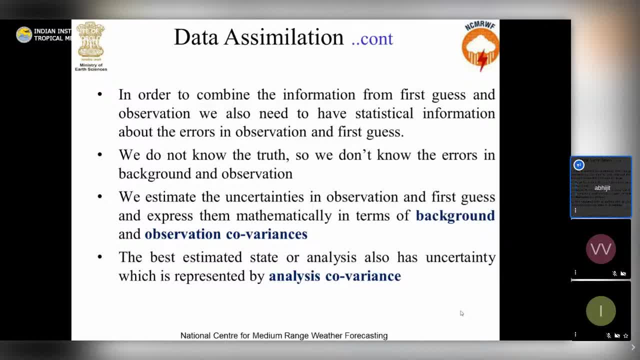 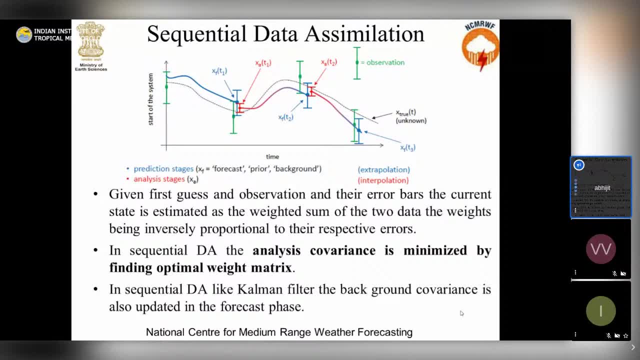 as analysis covariance, Sequential data in sequential data assimilation method, this analysis covariance. so it is, we try to minimize, We try to minimize. we give the weightage according to the amount of error associated with observation and first guess. So from a first guess, 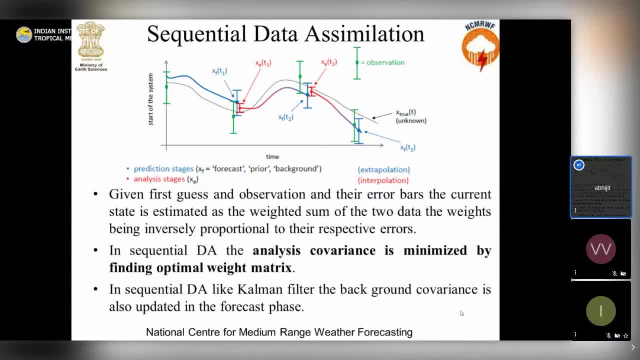 we run the model, We get that model forecast and we get the associated error. Then we compare with observation, which has also some error. Whichever error is more, the weightage is less, And from there we try to find out analysis. 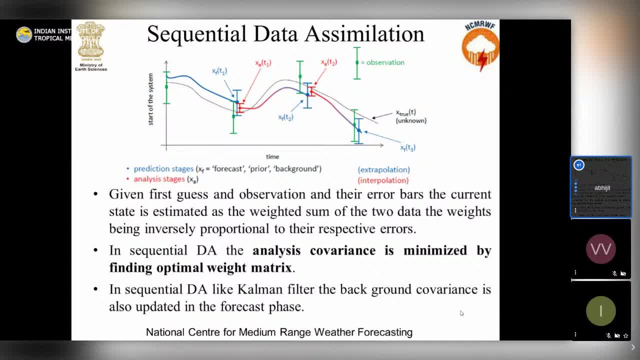 and analysis covariance by finding optimal weight matrix In the sequential data assimilation. like Kalman filter Ensemble, Kalman filter Ensemble transform, Kalman filter, extended Kalman filter. So these type of sequential data assimilation methods, not only these initial state, 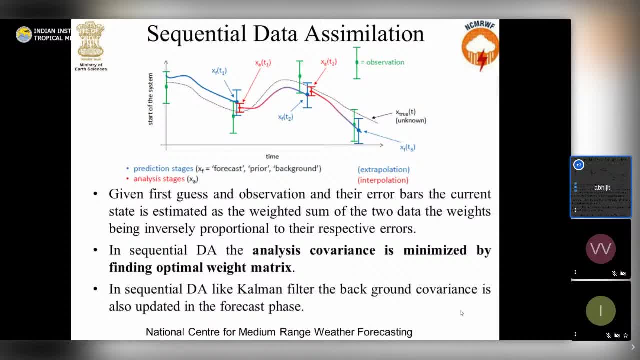 but also the covariance is also forecasted. So it has two stage. One is the prediction stage, another is the analysis stage. In prediction stage that forecast the state is model state is forecasted And in the analysis stage we find out the best estimated initial condition. 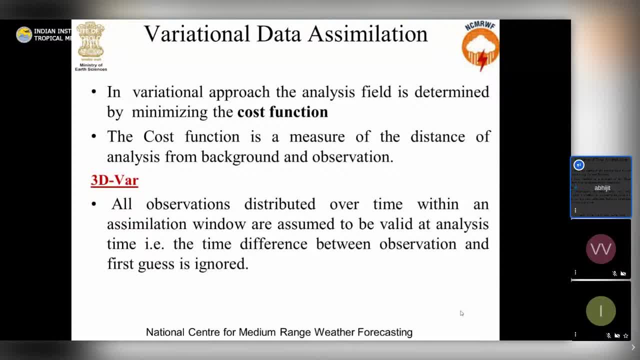 Next is variational data assimilation. In variational data assimilation method we try to minimize a cost function, which is type of a distance between both the first guess and the observation, And there are different types of variational data assimilation. 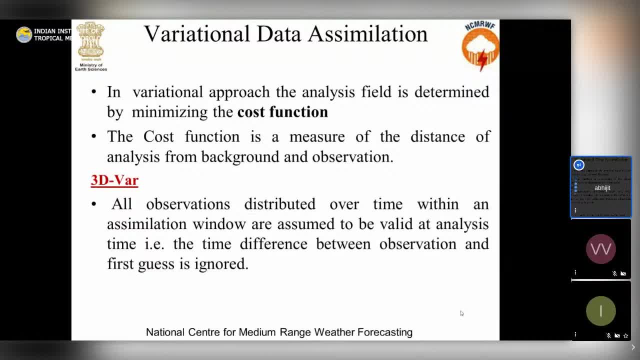 There is three-dimensional variational data assimilation. Here we assume that all observations which are actually distributed over the whole time window, so they are valid at the same time, although it is not true. So that means the time difference between observation and first guess. 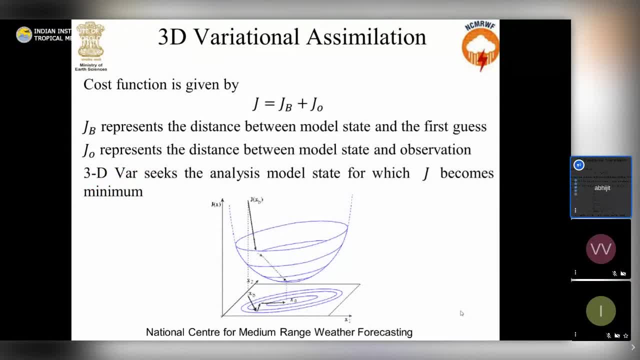 that is ignored. So this cost functions. so it has two parts. One is the background cost function, another is observation cost function. Background cost function JV represents the distance between the model state and the first guess And this observation cost function JO. 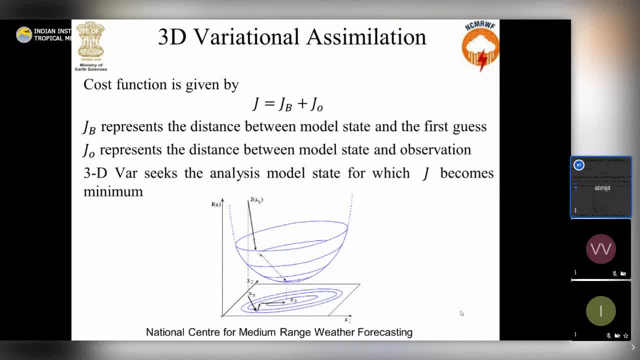 it represents the distance between model state and observation And through 3D VAR we try to find out that model state which will give us the minimum cost function. In this below figure we can see that we are looking for that model state. 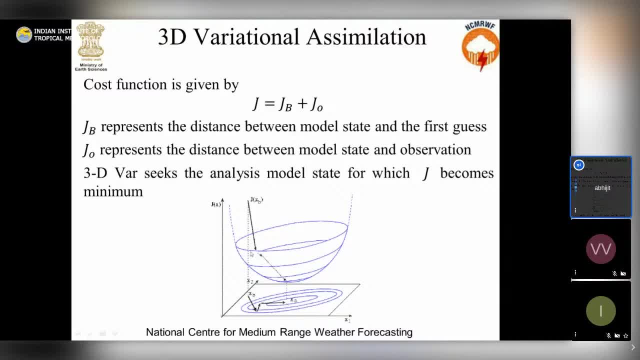 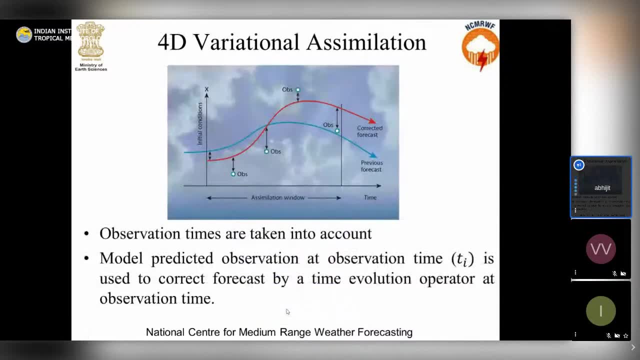 or that wheel for analysis for which we will get that cost function is minimum. Whereas in three-dimensional variational assimilation we ignore the time factor, in four-dimensional variational assimilation we take into account the time Because the observations are distributed. 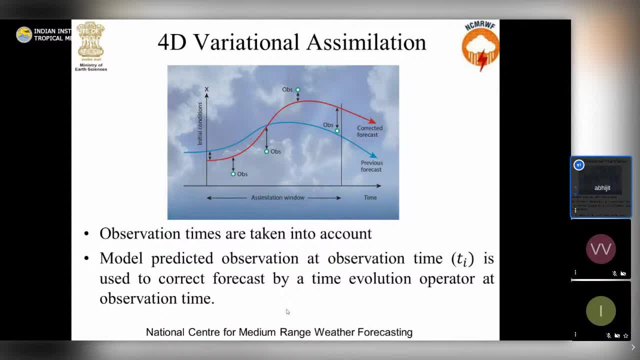 over the whole time window. so through a tangent linear model we try to forecast these observations. So from a first guess we try to forecast at the observation time what is supposed to be the model state at the observation time, And then we correct the whole trajectory. 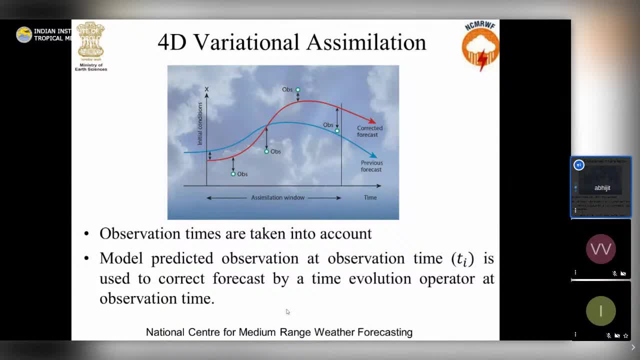 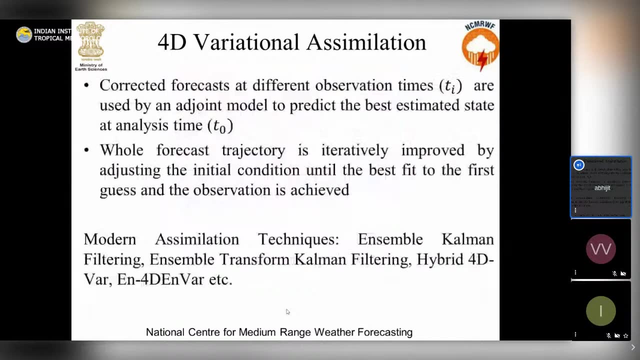 of this forecast, this iteratively, and we try to find out what will be the value of the first guess when this trajectory is best fit with the observation and the first guess. So corrected forecasts at different observation times are used by the adjoint model. 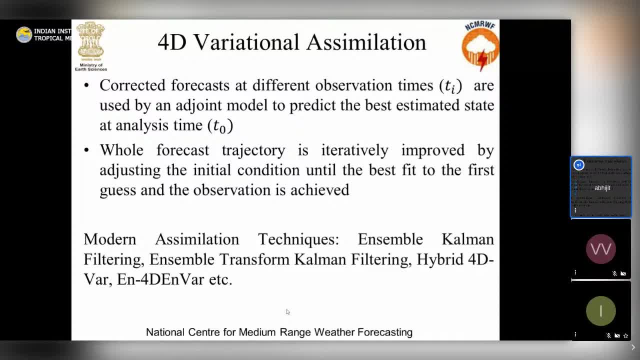 to predict the best estimated date at the analysis time. And the whole forecast trajectory is here iteratively corrected by adjusting the initial condition until we get the best fit for the first guess and observation. But these modern assimilation techniques, they take care of both the systems. 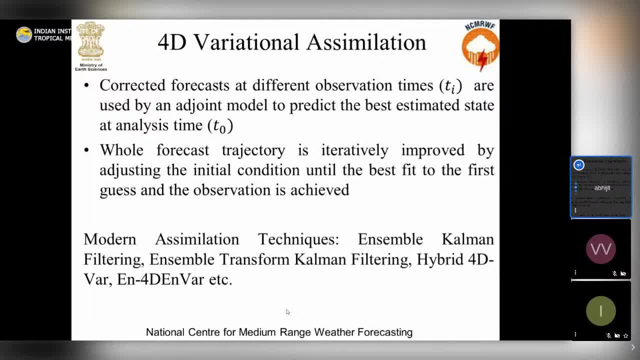 both the sequential assimilation system, which where the background covariance matrix is subflow dependent, and also these variational assimilation systems, where these background covariance are static. So the modern assimilation techniques are: ensemble Kalman filtering, ensemble transform Kalman filtering, hybrid 4D VAR, ensemble 4D, ensemble 4D VAR. 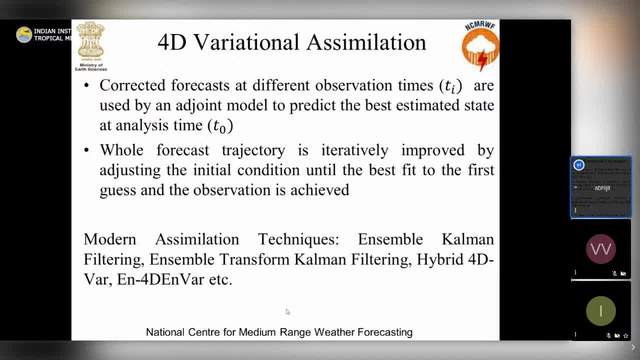 So these are the different assimilation techniques. Now, at the end of these data assimilation techniques, what we will get? We will get one physically consistent set of data set, or physically consistent initial conditions, where all the variables, they are physically consistent with each other. 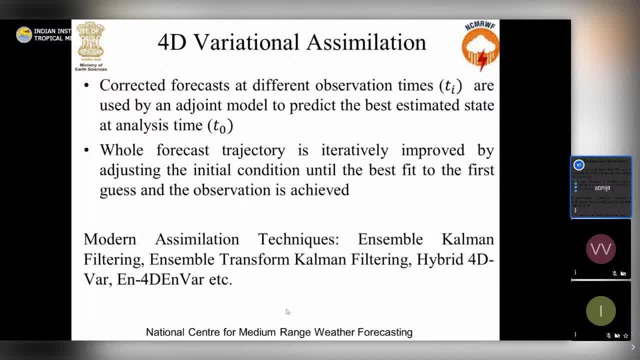 And generally we try to remove these high frequency waves, inertia, gravity waves, from the initial conditions so that so those frequency, those waves cannot create any noise in the short range forecast. Because if our short range forecast become bad, so then our first guess also will become bad. 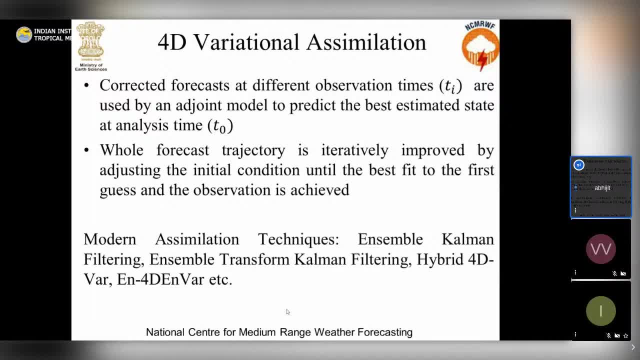 So it takes some spin up If we don't remove those high frequency short waves from the initial conditions. maybe with time we call it spin up time, So these waves will be removed but our short range forecast so that will not be noise free. 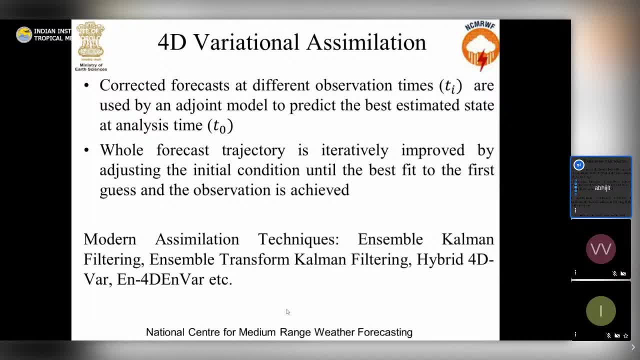 And, in general, these modern assimilation techniques. they remove these high frequency short waves from these initial conditions. So once these initial conditions are prepared by these modern techniques of data assimilation, so then we have to see how these governing equations can be solved. 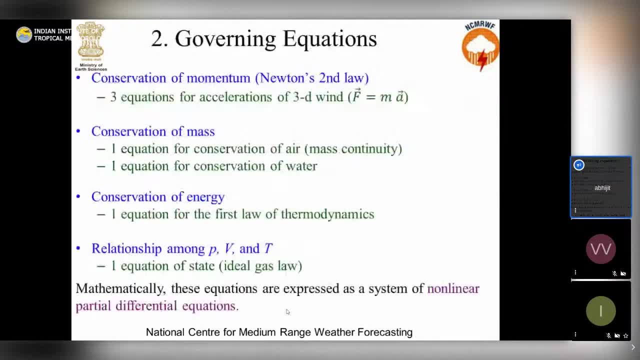 and what are these governing equations? So next is governing equations. These governing equations include conservation of momentum, which are the three equations for acceleration along the three coordinate axis, that is, east-west direction, north-south direction and these up-down direction. 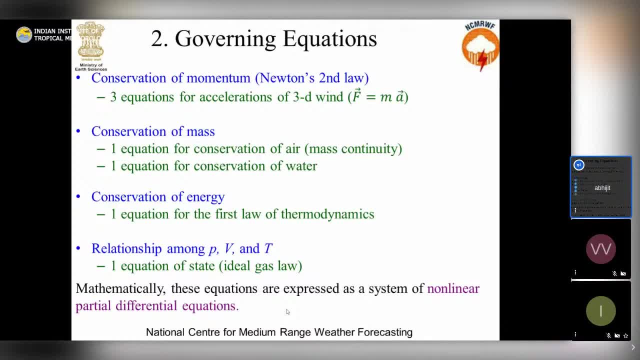 Then conservation of mass. There are two conservation of mass equations are used: one equation for conservation of air, another equation, separately, for conservation of water. So, because water is an important component of this atmosphere, it is not only that, because that we are very much interested. 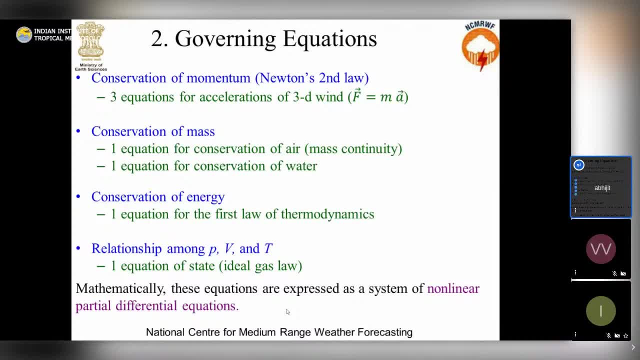 for this precipitation forecast. but also water is the major component which transports heat and moisture from one level of the atmosphere to another level. And then we solve conservation of energy equation. that is here. energy means we take care, only heat energy. So that is the first law of thermodynamics. 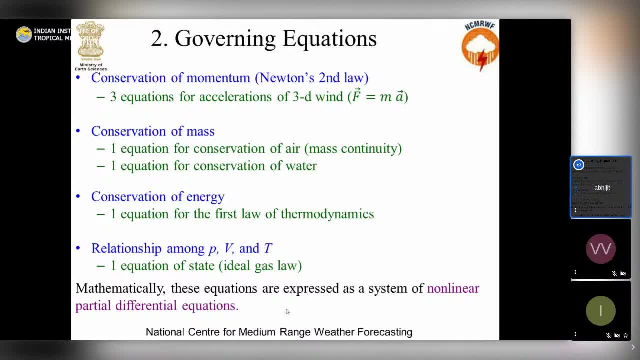 and the relationship among P V T. So that is the equation of state. These equations are non-linear, partial, differential equations. So these equations we cannot solve it by analytical method. So we have to solve these by numerical methods. That's why this modeling is called 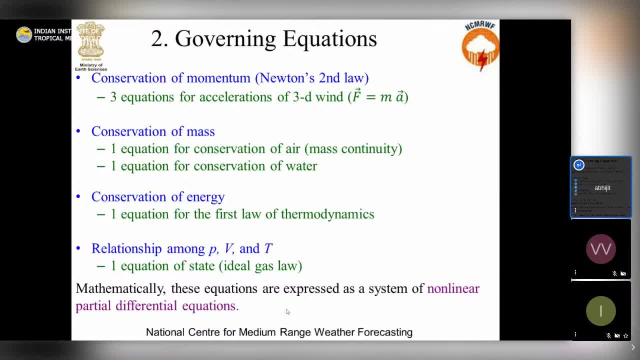 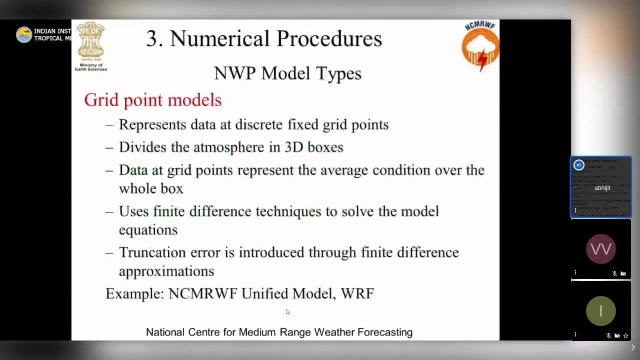 numerical modeling And, moreover, the computers can operate only these four arithmetical operations, that are, addition, subtraction, multiplication and amplification. And there are two types of models, that is, grid point models. In grid point models the data are represented. 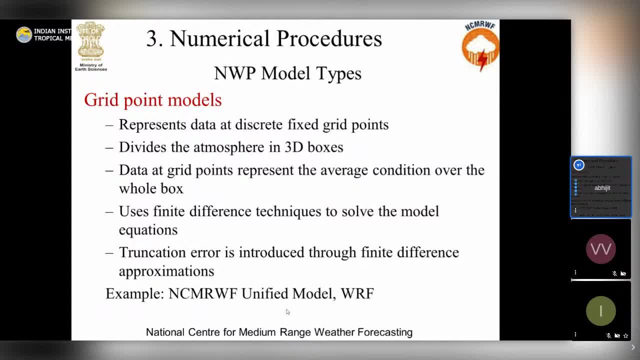 at discrete, fixed grid points And actually it divides the atmosphere in three-dimensional boxes And data at each grid point so that you present that whole box of grid points. So this is the grid point model. So this is the grid point model. 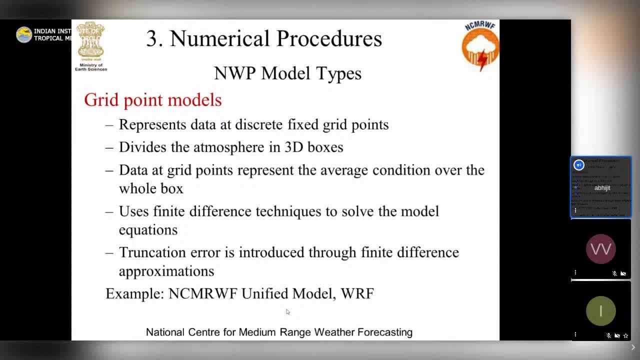 This is the model box average value of the variable, Not necessarily that always this grid point should be at the corner of the grid boxes, So it depends on the which staggered grid we are using so that, depending on that, that grid points location. 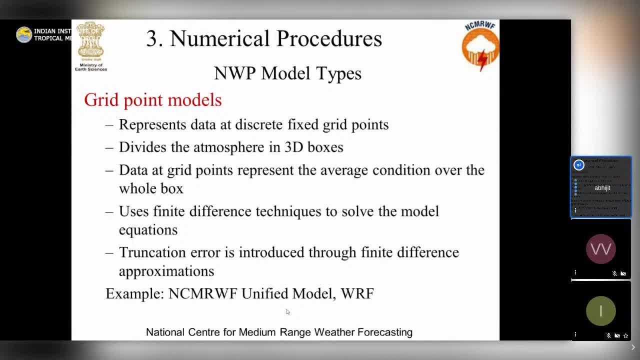 will be placed in a box. It uses finite difference technique to solve the model equations. So that means we use Taylor's expansion series And that error associated with will be truncation error. So truncation error will be introduced through finite difference approximations. So just I am briefly recapitulating that till now. 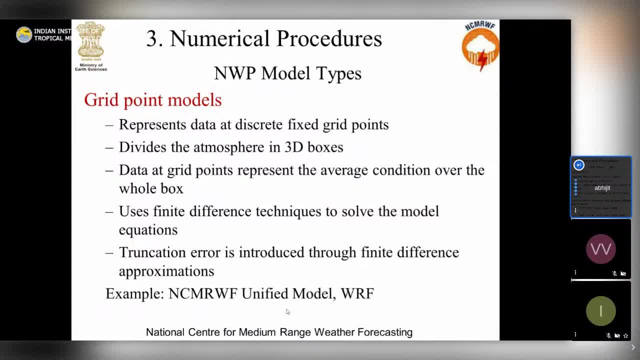 what we have discussed. So that is first that we discussed about these. preparation of the initial conditions. We have prepared the best estimated state of the initial conditions but it is not the true state. So that means some uncertainty or some error. it is associated with our initial. 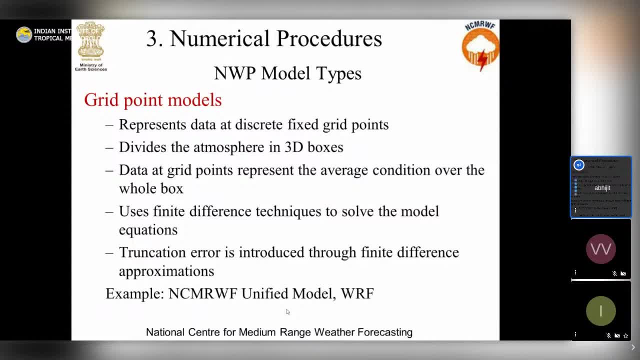 conditions. Then we have formulated the model equations. The model equations also are not free of errors, So different types of approximations are taken in different terms. So in the formulation of the model equations also the uncertainties are associated with it. And then when we are dividing that whole, 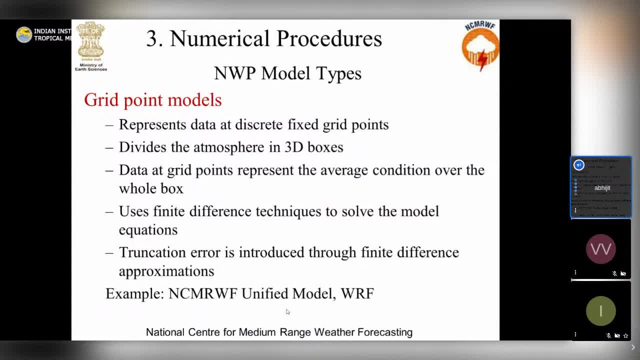 atmosphere into boxes and we are using Taylor series. that means we are removing these higher-order terms of the Taylor series. we are incorporating some error in this method Now. example of this grid point model is NCMRW unified model and WRF model, weather research and forecasting model. 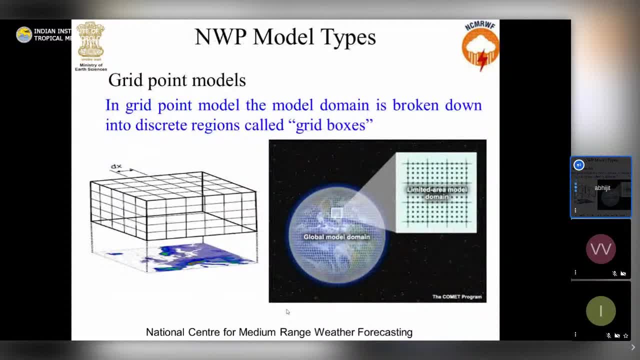 And there is another type of so this. you can see this grid point model here. so it is showing that how the atmosphere is divided into grid boxes. There are two types of model domains are shown here on the right side that is. one is global model domain, another is limited area. 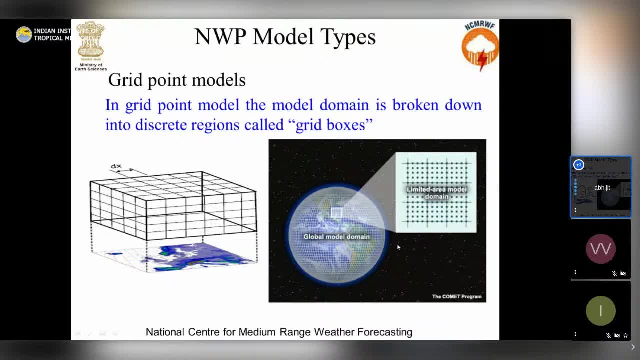 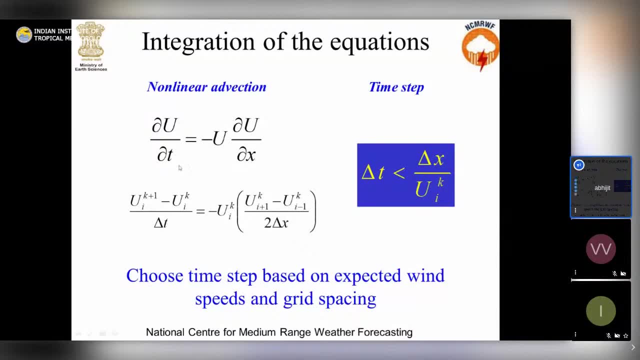 model domain. I will talk about this limited model area model domain later. And if we take this equation, this is non-linear advection equation. So, since it is the product of two dependent variables, one is u and another is del u, del x, so this term is called the non-linear term. 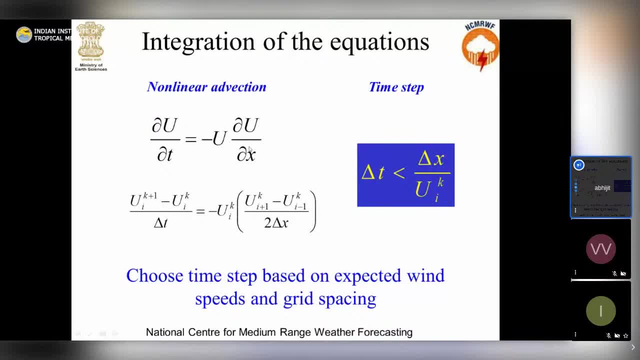 So this is a differential equation. we are converting this differential equation, or a problem of calculation, into problem of algebra. So here these operations are only the subtraction, addition, multiplication and division, and this delta t, so it is giving the time step, so it is not the 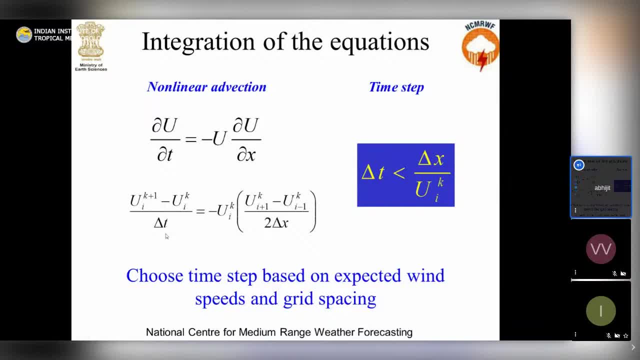 continuously. we are progressing with the time. so we are progressing with the time discreetly. and this delta t we cannot take as much large as we want because we have to follow some condition. this is the essential but not sufficient condition for that: how much we can take delta t. 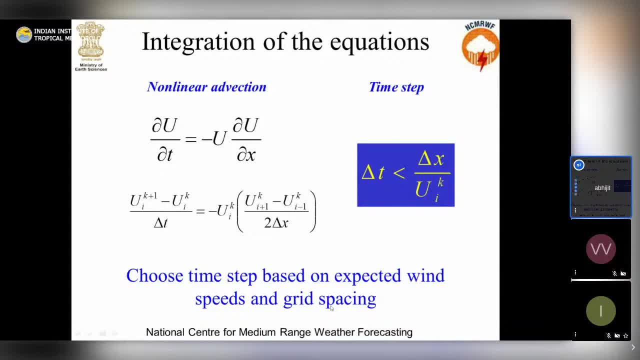 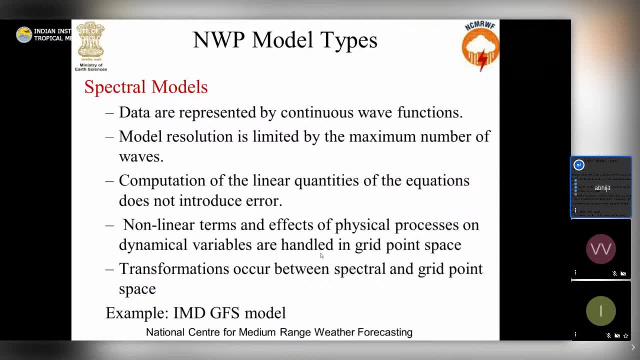 So this delta t will be according to the wind speed and grid spacing. And then another type of model in spectral model. so in this spectral model this data represented by continuous wave function, so it is the linear combinations of different waves of different wavelength, So it has to be a linear combination of various waves of different wavelengths. 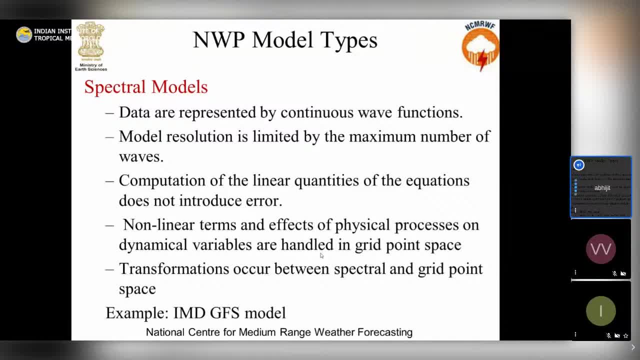 and model resolution is limited by the maximum number of waves. so how many maximum number of wave we can accommodate according to our resources? so that will decide what will be the resolution. and this computation of linear quantities of this equation does not introduce error, so they will be properly calculated. but the non-linear terms and then the physical processes. 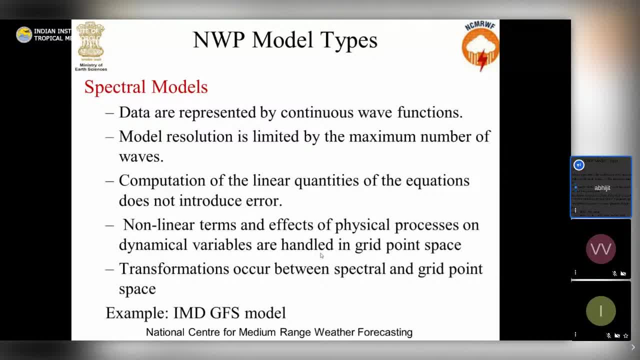 and these also this vertical advection term. so those terms, they will be calculated in the grid. so frequently we have to transform from the spectral space to the grid space and while transforming from the spectral space to grid space and vice versa. so there will be some error. and whereas the taylor series is used in grid point model, in these spectral models the 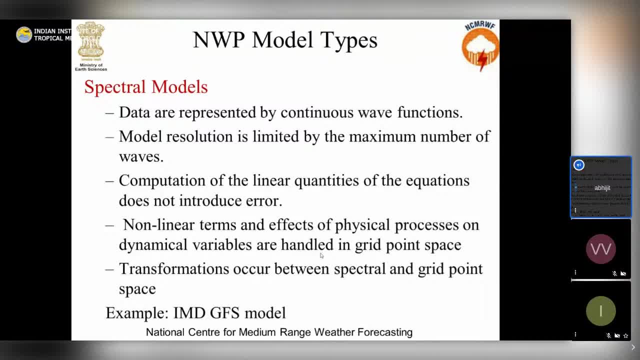 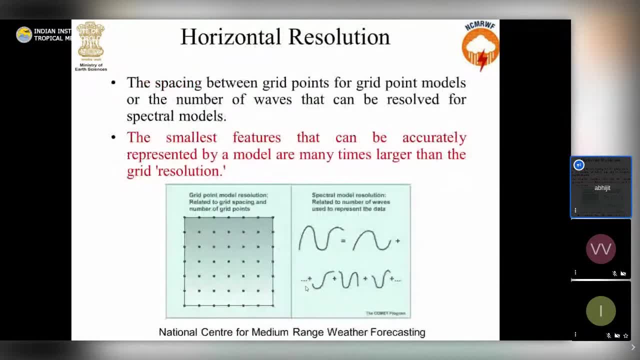 series is used and imd gfs model is one example of spectral model. Now what do we understand by horizontal resolution? So the separation between the two grid points in a horizontal plane. so that will give us the horizontal resolution in a grid point model. So if we take this, 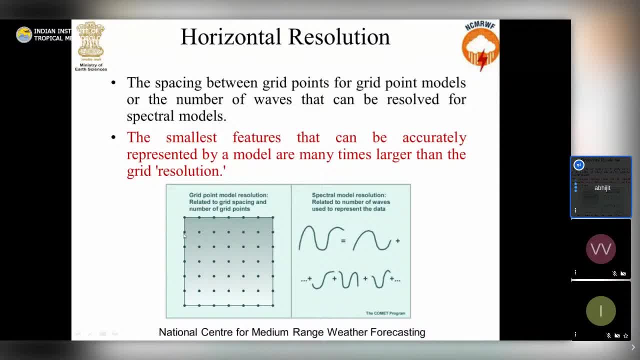 is as the x direction and this is as the y direction. so this delta x, that is the separation between the so consecutive two grid points, so that will give us the horizontal resolution of the model and in a spectral model, so that will be the smallest. that will be decided by that how many maximum number of 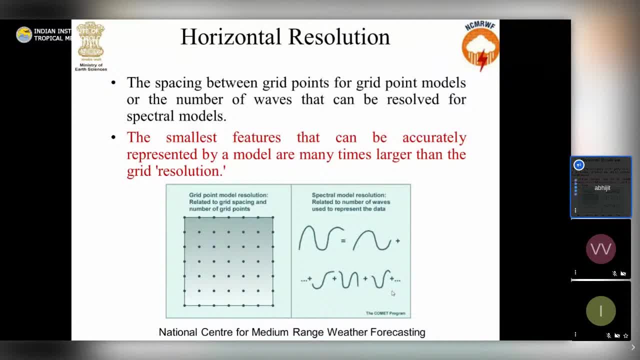 waves we can or what that we can resolve, But it is different from the smallest feature that we, that we can resolve by our model, because we need at least five to seven grid points to resolve a phenomenon, So the smallest feature that we can resolve, so that will be much, much larger than these grid spaces- Then vertical, 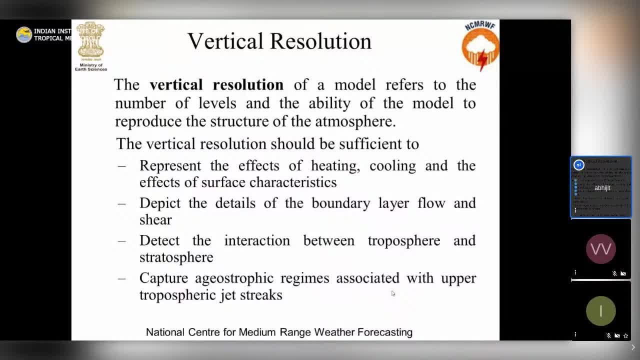 resolution. it means that what is the separation between the vertical levels? that the vertical resolution should be sufficient to represent the effects of heating, cooling and these other surface characteristics, and it should be able to depict the details of the boundary layer flow and other boundary layer phenomena. and so means the vertical resolution should be. 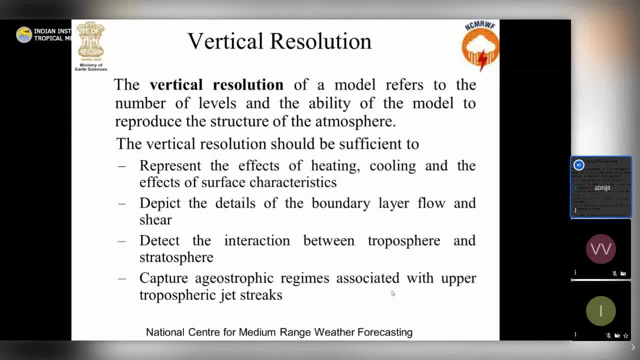 high, where the gradient will be very large, but at the same time at the upper toposphere or above 500 HP. also, we need a sufficient vertical resolution to resolve the interaction between toposphere and stratosphere and also to capture a geostrophic. 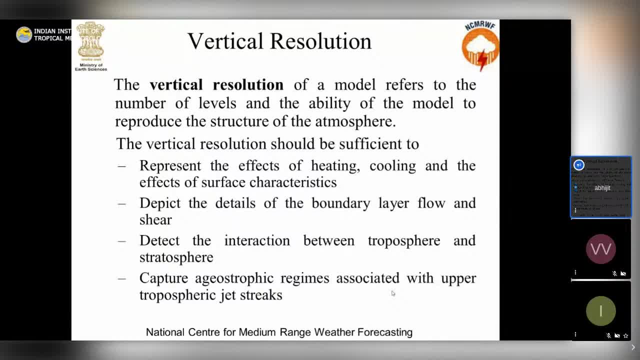 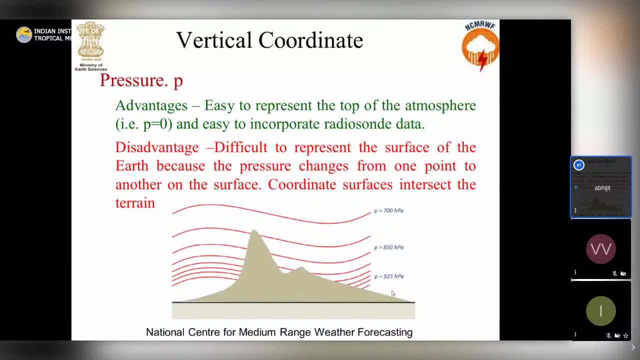 designs associated with topospheric jet streaks. Different types of vertical coordinates are used to for this model, to construct a model. So most easy is that a z coordinate or height coordinate. Height coordinate is very easy to construct and very intuitive. but problem with the height coordinate is that your 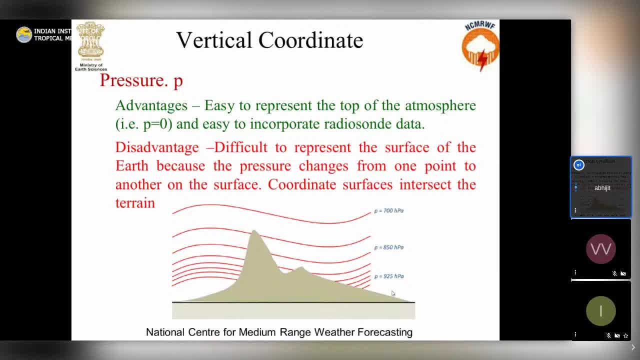 z is equal to constant, does not always give us the lower boundary or the surface of the earth. So we an atmospheric flow. it depends on. the flow is governed by the special gaudians, so we can take the pressure as the vertical coordinate. and again, its advantages is that it is easy to 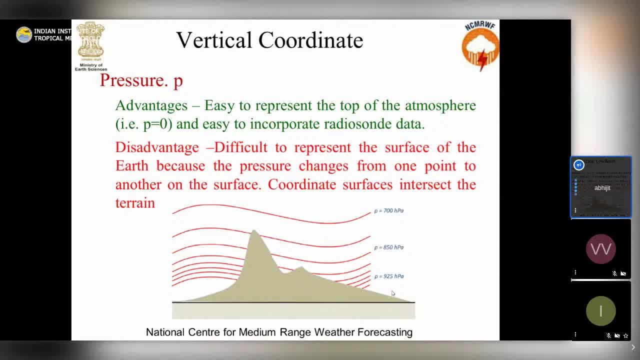 represent the top of the atmosphere and it is easy to incorporate, reduce on the data if we take the pressure as the vertical coordinate. but again, like z coordinate, the vertical pressure coordinate also has that disadvantage that it can cut the terrain, Difficult to represent the surface of the earth because the pressure changes from one point to 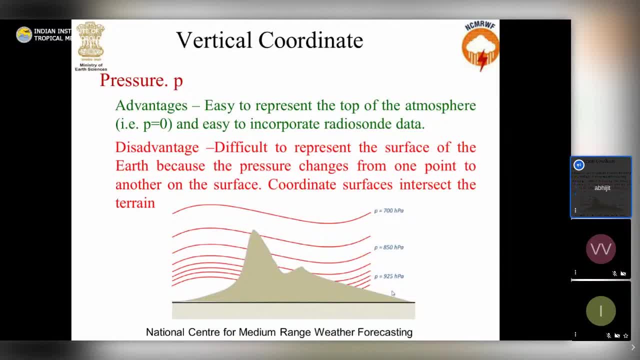 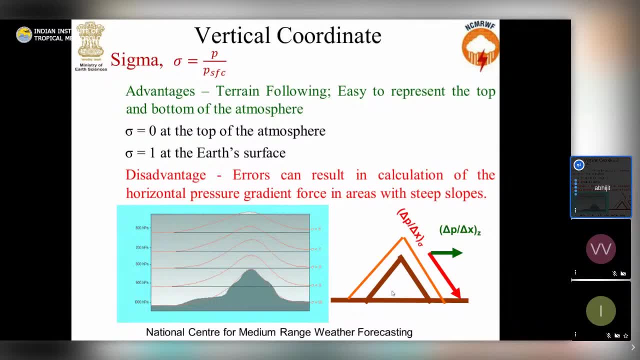 another on the surface. We can take a terrain following coordinate system. that is sigma. So it gives by pressure at an 11 divided by the pressure at the surface and sigma is equal to 0. So that indicates the top of the atmosphere and sigma is equal to 1. It indicates the earth surface. 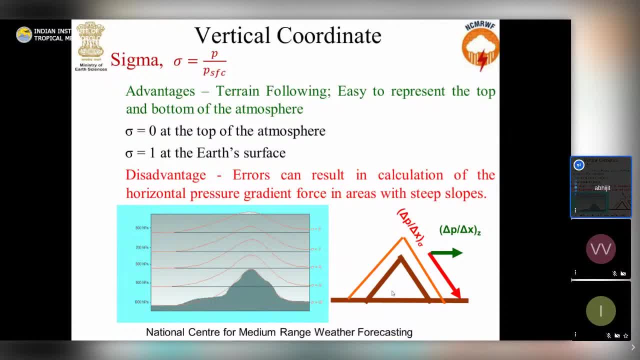 Its disadvantage is that it cannot properly represent that horizontal pressure gradient 4 star, and also it makes the terrain very smooth. So in that case, like on the lee side, that cold air damming, those phenomena are not being properly represented by the sigma coordinate system. 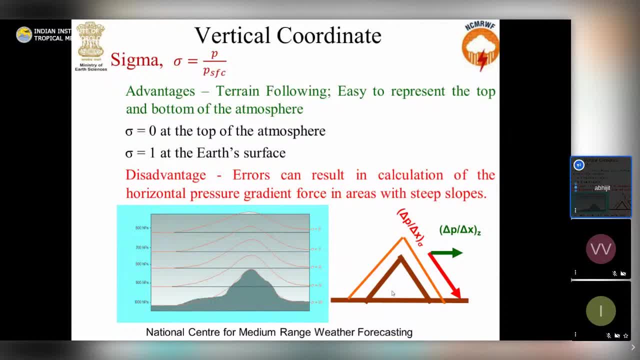 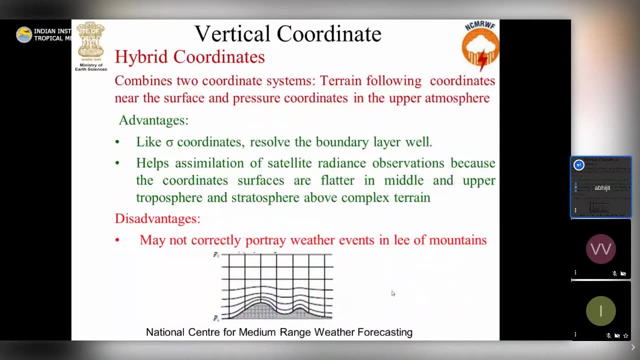 So all these these pressure coordinate systems, sigma coordinate systems, so they have their own disadvantages and advantages. but in the modern numerical weather, northern numerical models, So generally the hybrid coordinate system is used. in this hybrid coordinate system, At the lower atmosphere we use the sigma coordinate system and at the upper atmosphere we use 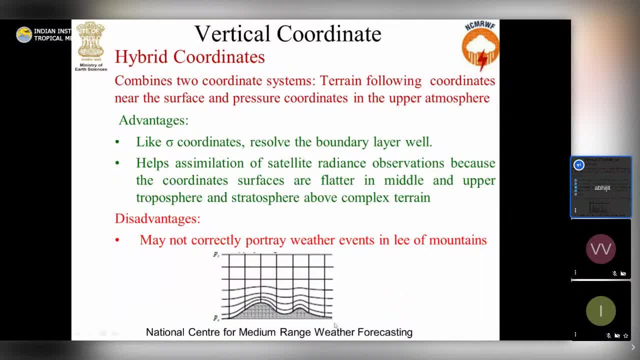 pressure coordinate system which is very flat. So we can see that in this figure that in the lower atmosphere it is, it is the terrain following sigma coordinate system. where is the upper atmosphere? it is the fat pressure pressure coordinate system, pressure coordinate which helps in assimilating the satellite radiation, of radiance of surface. 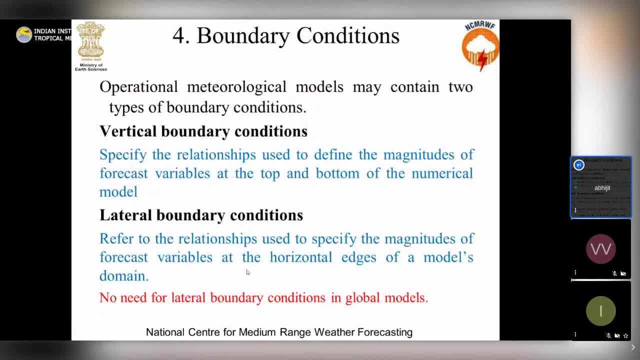 Next comes boundary, boundary conditions. Now, in actual atmosphere we have only one boundary, that is the lower boundary, which is defined by the earth surface. but when we try to model this atmosphere we have to compute within a finite time. So we have to put some artificial top boundary. So we need two boundaries, at least two boundaries in the 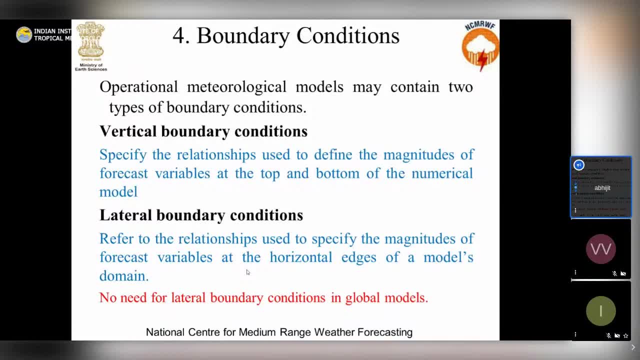 model. So in the global model there are two vertical boundaries: one is the lower boundary, another is the top boundary, And if we consider about the regional models, so then we have to artificially direct four lateral boundaries. So then this lateral boundary conditions refer the relationship used. 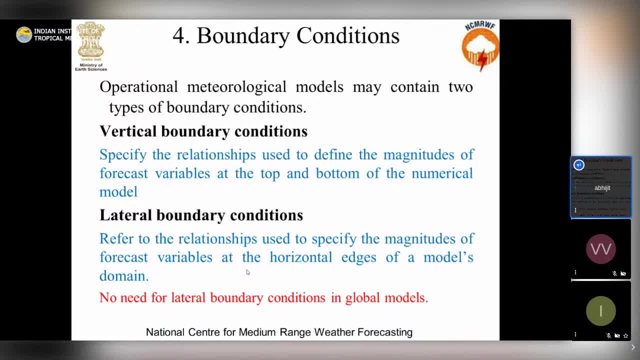 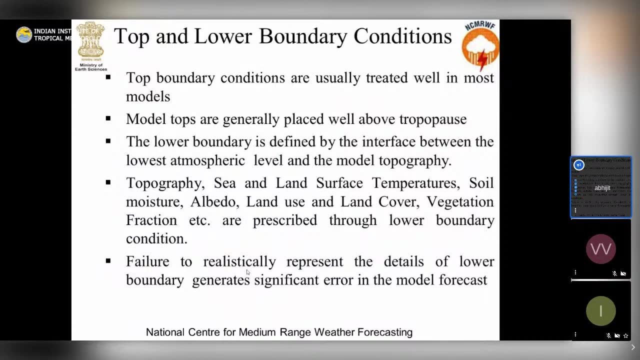 to specify the magnitudes of forecast variables at the horizontal agents of the edges of the model's domain. But global boundary does not need any lateral boundary condition. Now the boundary conditions do not give much error, so model tops are privately placed Well above the toposphere. it is like our, that NCMWF global model, that the top boundary 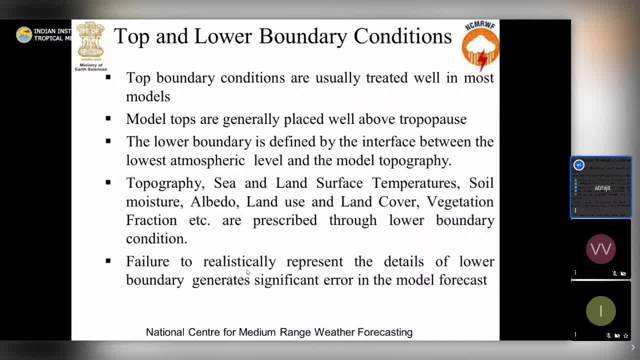 is located at about 70 Kigueh meter height. The 80 kilometer height and that lower boundary is defined by the interface between the lowest atmosphere level and the model topography, And now we can see that of an atmosphere range like that. 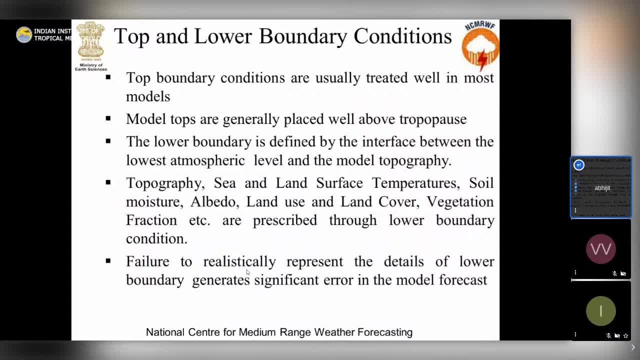 So the lower boundary. it contains this topography, then sea and land surface and then the many variables we have to specify accurately in the lower boundary. but because of the finite resolution of the model we cannot totally replicate the lower boundary within the model. 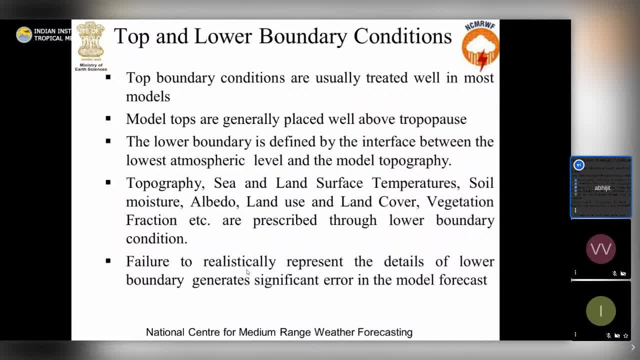 So we have to. we have to somehow model these lower boundaries also, so that errors are not more. but the error is inevitable through the lower boundary which we will be going into the model. So failure to realistically represent the details of lower boundary generates significant errors. 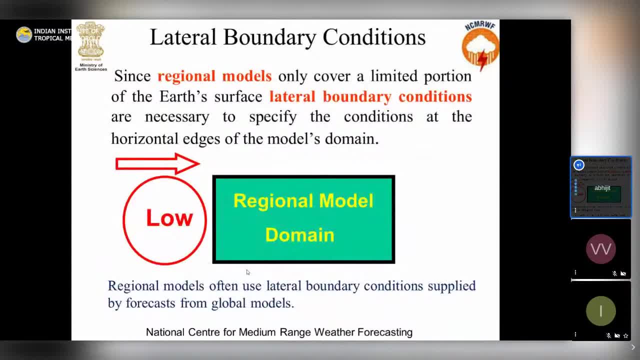 Then comes lateral boundary, While we were talking about regional model and we know if we consider about the grid point model. so then you have to hydrate our atmosphere into grid boxes Now, the grid box, which is very much interior within this model domain, so it gets the information not only from within the same box, but also from these. 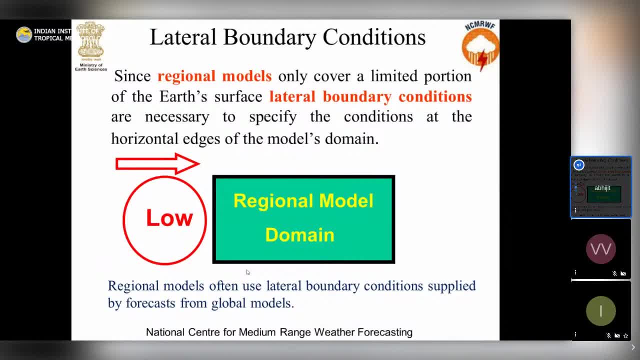 surrounding neighboring boxes, But the box which is near the lateral boundary. it will not get the information from all the sides if the lateral boundary is rigid. So we have to make the lateral boundary transparent so that it can always communicate with the outside environment or outside atmosphere, so that information from the outside atmosphere it reaches the grid box. 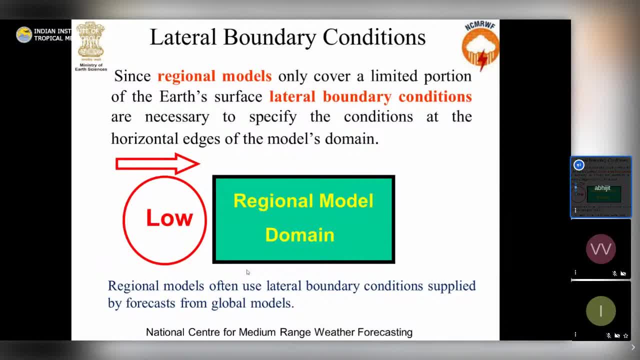 So regional models often use these lateral boundary conditions from these larger models or global models, But the it is not possible to give this lateral boundary condition at every time step. So what do we do? We give the lateral boundary condition after some regular time interval, which is the integral. 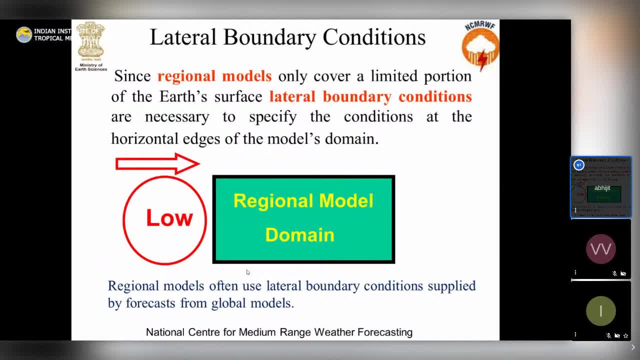 multiple of the time steps And suppose if we give, if our time step is only one minute, but if we give this lower lateral boundary condition every three hours, So we have to inter correlate this lateral boundary condition from 0 hour to 3 hour for every minute. So that will incorporate a lot of error in specifying the 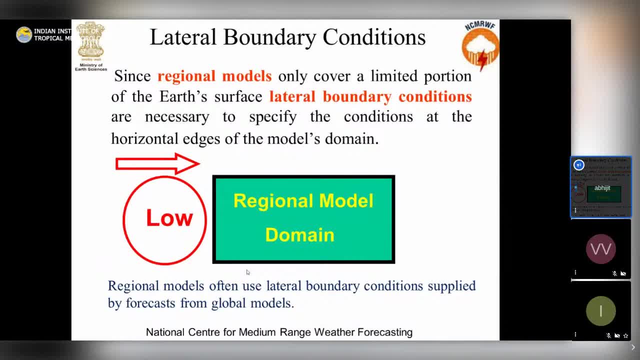 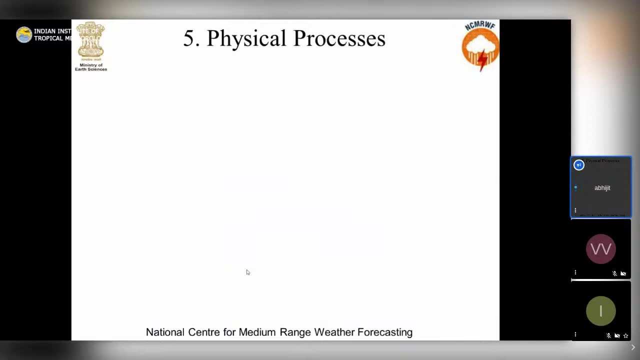 lateral boundary conditions. So the errors will come into the model through the prescribing the lateral boundary conditions and also prescribing the lower boundary conditions. corner commission series. User control, care of the physical processes which appear within these governing equations through source and symptoms. And these physical processes, most of the time they are sub-grids. They are so. 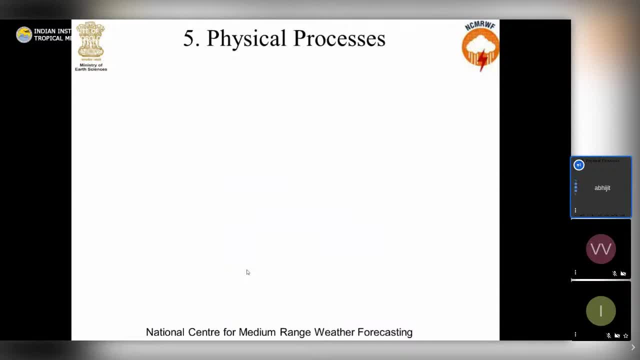 small, so that one grid cannot resolve these processes, But their effect on these large-scale phenomena, so that effect is significant. So what we do? We try to model the effect of these sub-grid scale processes statistically, sometimes by some assumptions, or sometimes based on some. 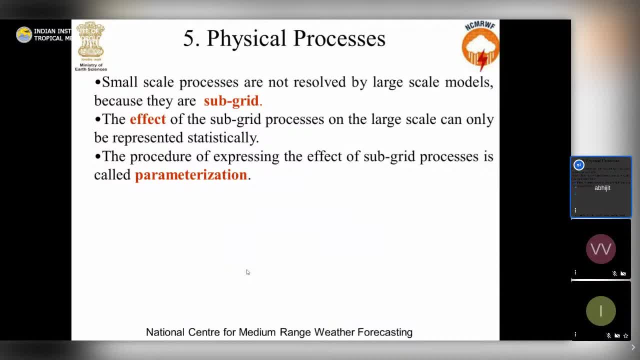 physical principles. So the procedure of expressing the effect of the sub-grid process is called parameterization. So first thing is that the sub-grid processes, it should derive their input from the large-scale phenomena. So then the sub-grid processes. we have to model the effect of these sub-grid. 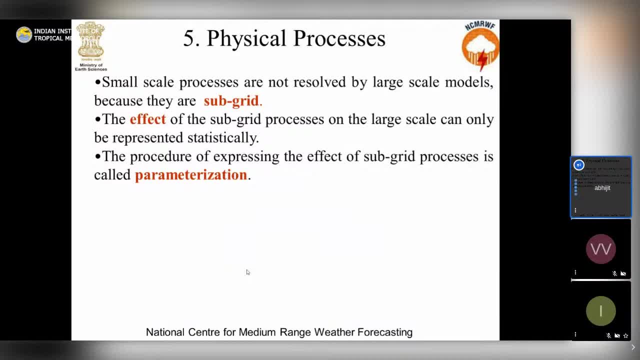 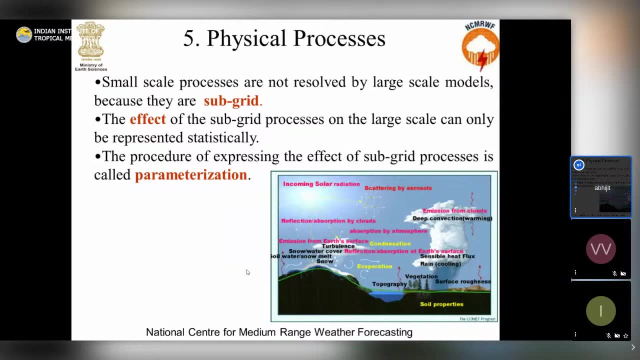 processes and then we have to express in terms of the large-scale variables. So these lot of uncertainties will be associated with this whole process of parameterization. These are the processes which we try to parameterize. So these processes include radiation transfer in surface processes, vertical turbulent process clouds and large-scale 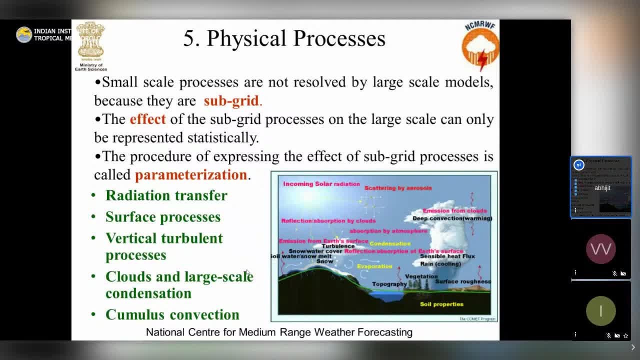 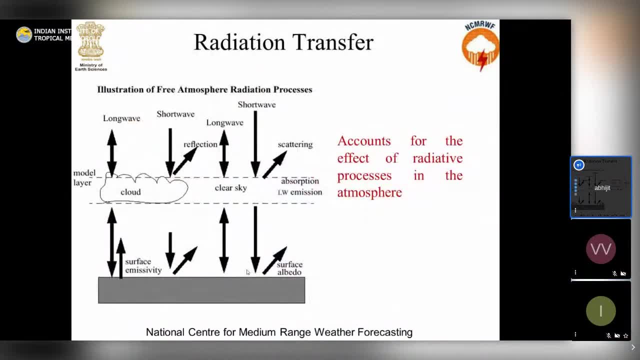 condensation, cumulus, convection. Now I will give a brief description about all these processes. Radiation transfer: it accounts for the effect of radiating processes in the atmosphere, How these radiation of different wavelengths, so how they are absorbed and reflected from different parts. 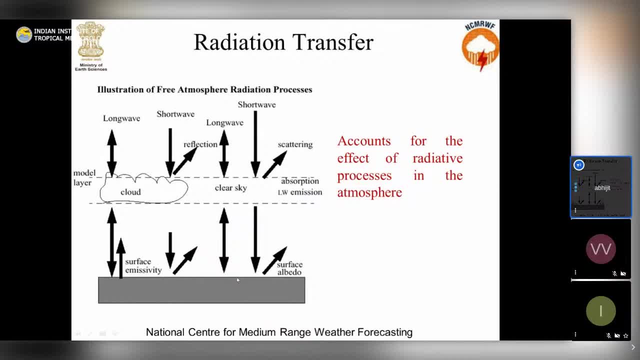 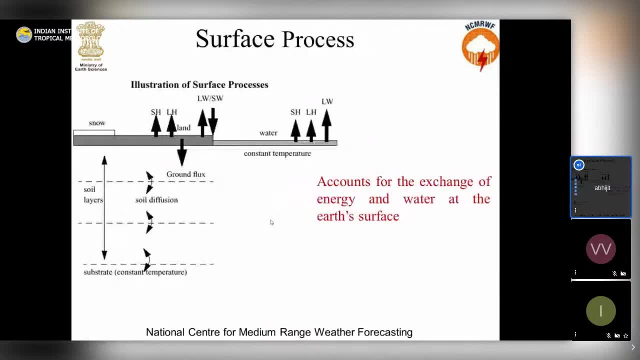 of the atmosphere and from the surface of the atmosphere. So we have to understand the effect of these atmosphere and so these are taken care in the radiation transfer. Then comes surface process, how the surface interacts with the atmosphere and it exchanges heat and moisture with these lower level, different soil levels. So these are taken. 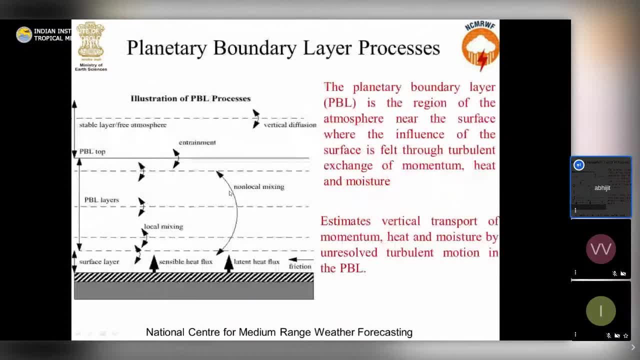 care in the surface processes, Then we take care, then we take care of the planetary boundary layer processes within this planetary boundary layer parameterization, PPL parameterization, So which estimates the vertical transport of momentum, heat and moisture by undissolved turbulent motions. 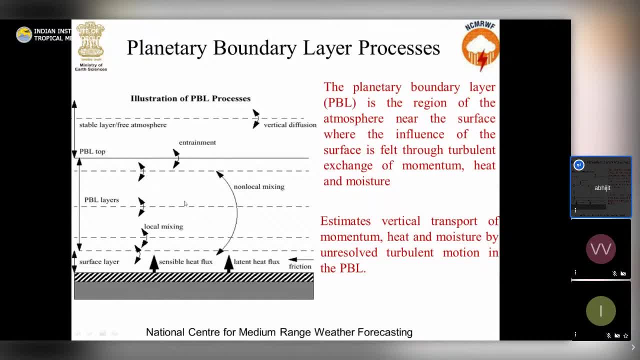 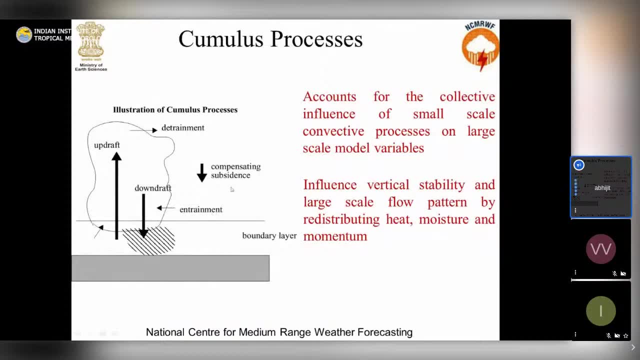 in the PBL, Then cumulus processes, so it accounts for the collective influence of small-scale convection processes or large-scale model variables. If our model has a large grid spacing and if the resolution is low, then we have to include one parameterization. 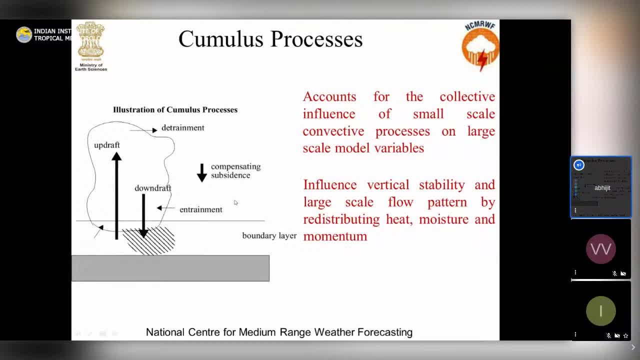 method for these cumulus processes. But if the grid spacing is very small or our model is of very high resolution, then the model will be able to resolve this explicitly, So we don't have to input any parameterization methods for these cumulus processes. 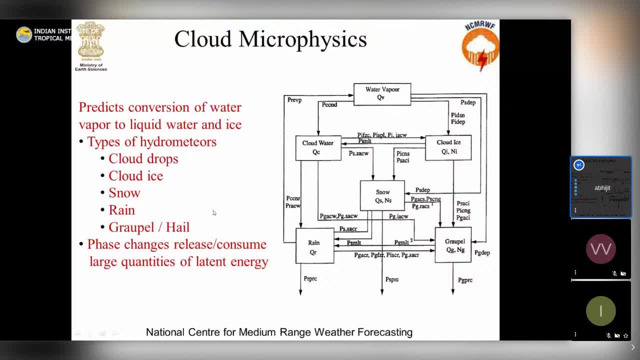 Then comes cloud microphysics, which predicts the conversion of water vapor to liquid water. So this cloud microphysics scheme decides this generation of the different types of hydrometeors, like cloud drops, cloud ice, snow, rain drop, L hail. So all these. 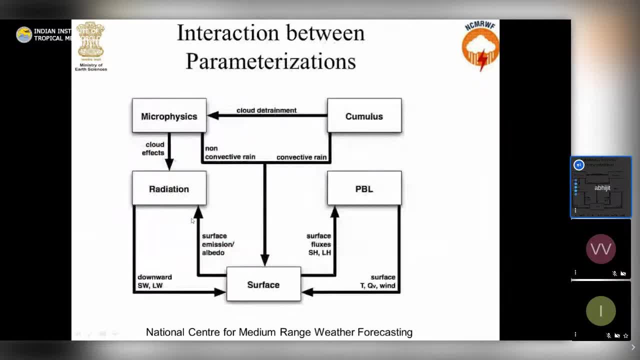 processes we try to parameterize and, moreover, these processes, they are interrelated with each other. So all these parameterizations, like cloud drop, rain, special snow and тому water, is interrelated with each other. So how much cloud this cumulus convection method will create? So that will. 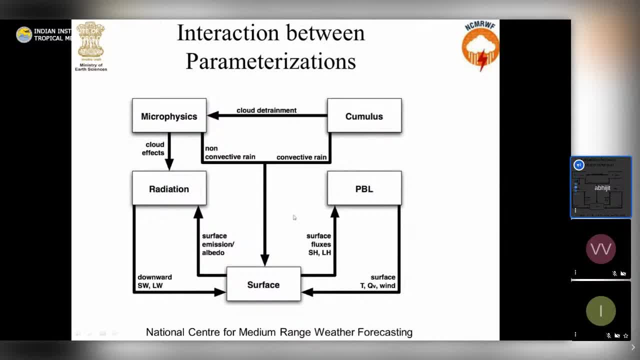 decide that, how much solar radiation will come and that will decide how much rain will be there. If there is some error in producing the cloud, there will be error in computation of incoming solar radiation or calculation of albedo, So then there will be problem in calculating these surface temperatures. 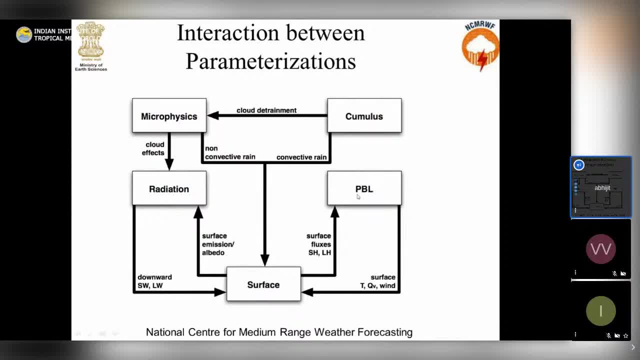 therefore, this cumulus convection will lately start to disappear. So we try to. So all these processes- PPL, surface radiation, microphytics, cumulus convection, all these processes, they are interrelated with each other. But since we are using parameterization, different parameterization schemes to take care of these, 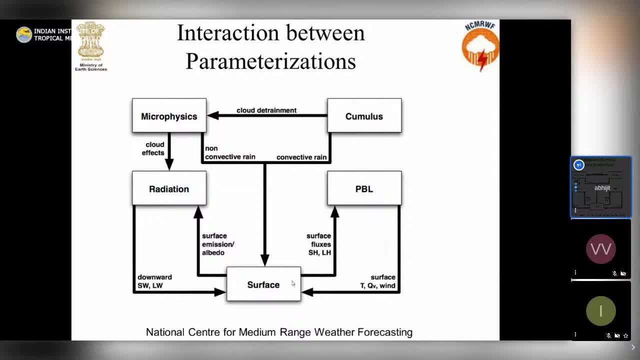 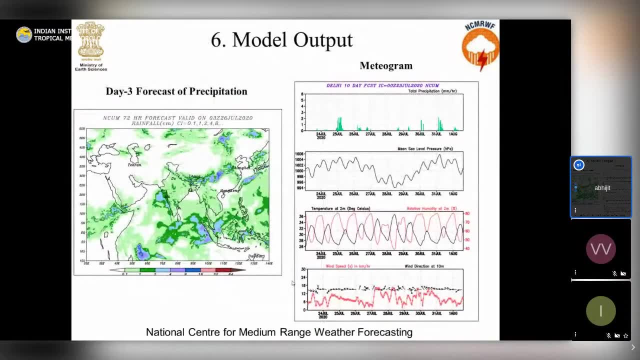 processes within the models. so there will be lot of uncertainties associated with the prescription of these processes within the model. And finally, we will create the model output. So we create, we produce this model output in the form of weather charts. So you can see on the left side this is giving the spatial distribution of rainfall from: 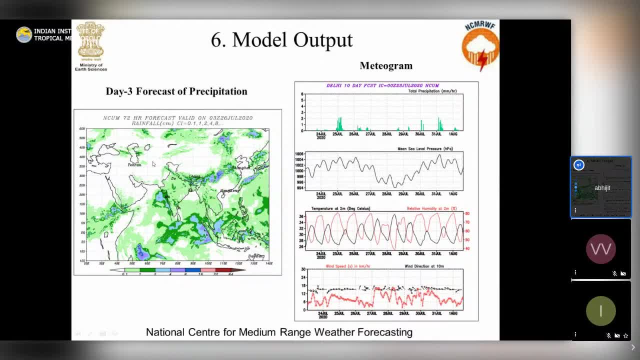 our NCRWF unified model, which is the 72 hours forecast how the precipitation is distributed. So it's valid on 26th July. So this way we will create the model output, We will give the precipitation forecast and on the right side we are giving these location. 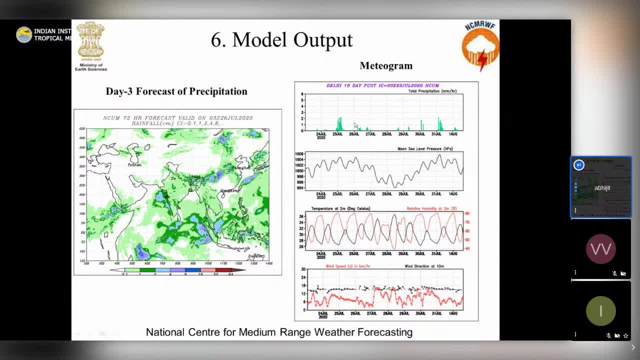 specific forecasts with the help of a meteogram. So the first panel, it gives the total precipitation. second panel gives the mean sea level pressure. third panel gives temperature and relative humidity and the fourth panel gives wind speed and wind direction. But when we are telling this, when we are expressing these model outputs with the help 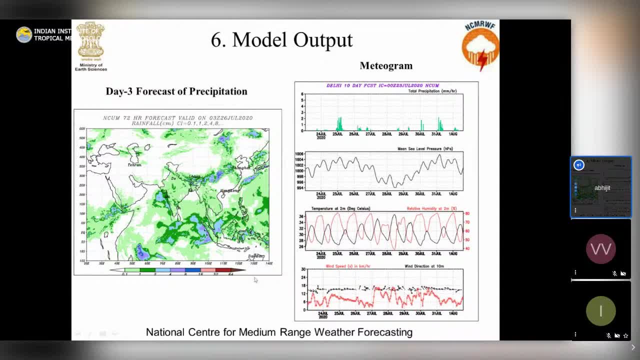 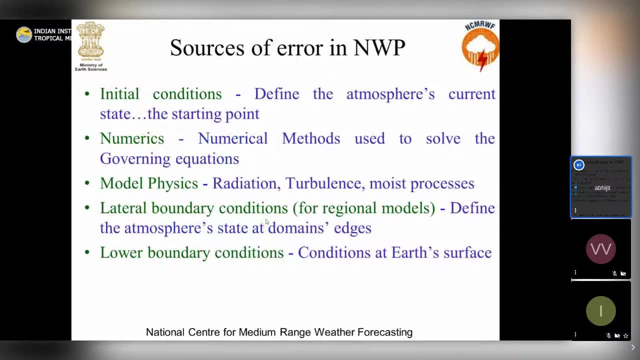 of these charts. We are not communicating any information related to uncertainty of the model forecast, As we have seen that at every stage of these NWP there is some uncertainty associated with it, Like in initial condition when we are defining the atmosphere's current state, when the method 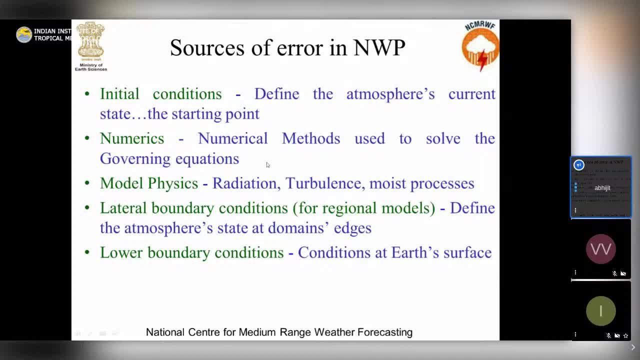 of solving these governing equations, Even the formulation of the model, Even the formulation of the model, Even the formulation of the model, also have some uncertainty. That parameterization of the physical processes, that also will have uncertainty. Describing the lateral boundary conditions, describing the lower boundary conditions, 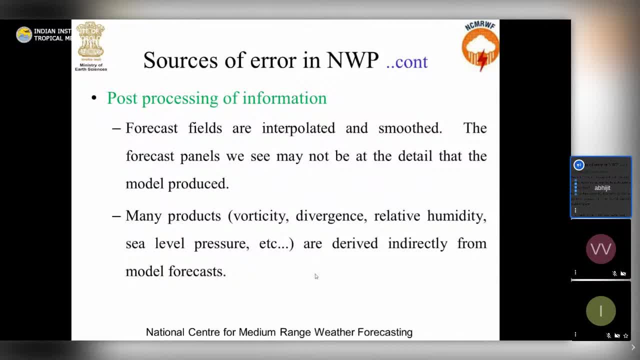 And when we are generating the model output, then also there will be error, because maybe we are interested with those outputs which are not the model variables. So we have to convert the model variables, So we have to convert the model variables To the desired output, like vorticity divergence, relative humidity, sea level pressure. 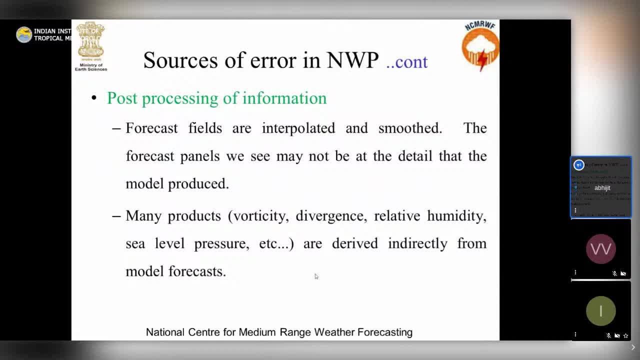 There are the derived quantities from the model variables And also suppose we want the model output at some location where we have to interpolate from the different grid points, the model variables. So there will be errors associated with the post processing of information. also We have to interpret all of them. 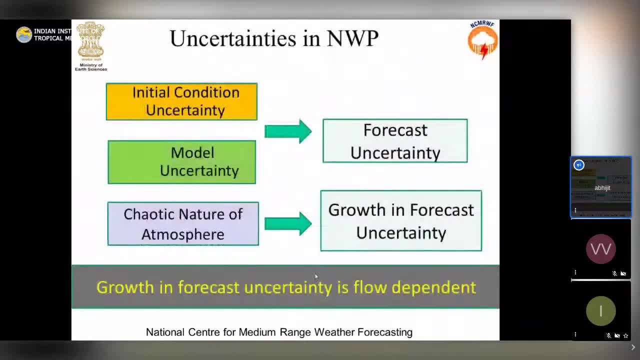 So we have to interpret the model variables. So we have seen that there is uncertainty associated with initial condition and there is uncertainty associated with the modern physics. So mainly these are the two big uncertainties: one is with the description of the initial state of the atmosphere and another is associated with the parameterization of the physical. 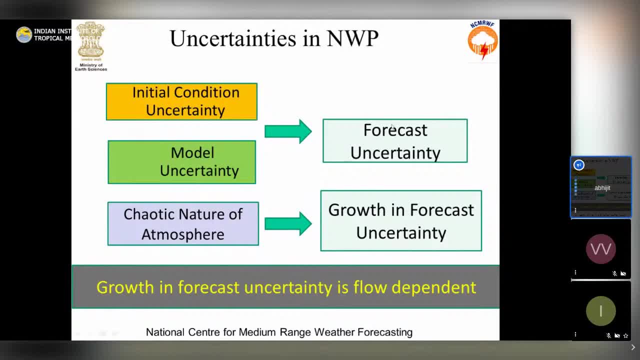 process which lead to the uncertainty in the forecast model forecast And we know that atmosphere is a chaotic system, so means that initial air condition uncertainty can grow with time. it can grow so fast that within a very short time it can make the model. 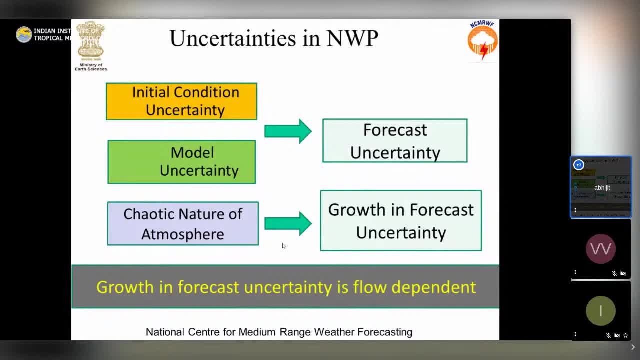 forecast useless. So it is not always the limitation of the forecasting system but it is the nature of the system itself. and again, that growth of the forecast uncertainty. it is flow dependent on different days, this growth of uncertainty, so that will be different. 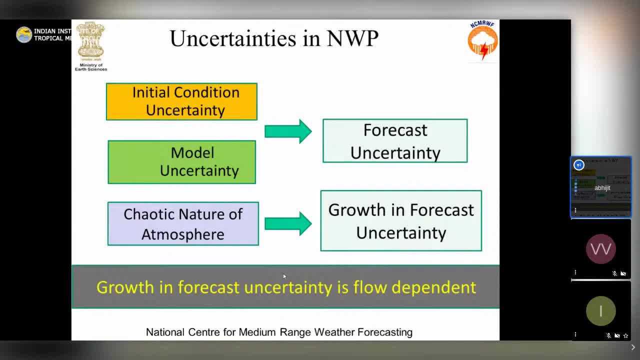 So we cannot beforehand that anticipate that. how much will be the growth of the uncertainty? So there is uncertainties associated with initial condition and modern physics atmosphere is a chaotic system and the growth of uncertainty it is flow dependent. So how the uncertainty will develop. 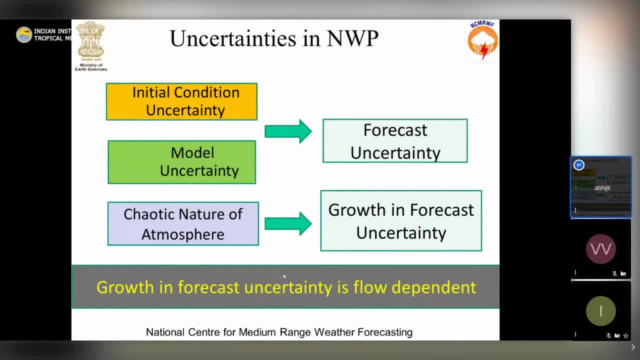 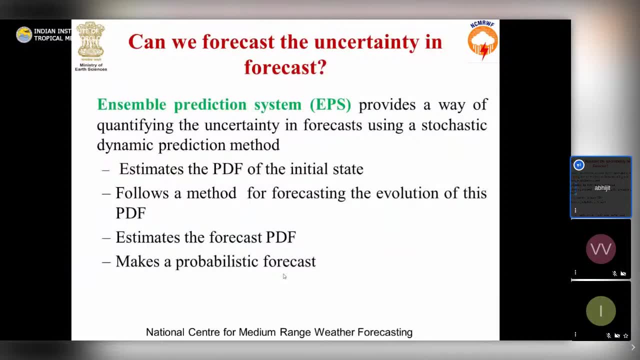 Let me summarize. So let me summarize: flow dependent. so question is: can we forecast the uncertainty which is associated with the forecast? so that will be very much useful for the users and the forecasters. so if, along with the forecast, if we can beforehand forecast, 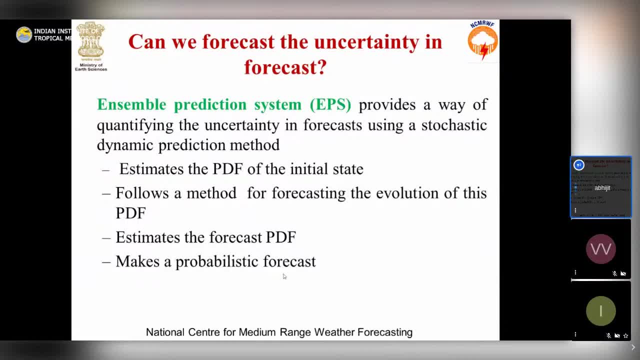 that how much uncertainty is associated with that forecast. so that will enable the users to take proper decision in sample prediction system. it provides a way of quantifying this uncertainty in forecast by using a stochastic dynamic prediction. so what we do by stochastic method or by statistically, we find out. 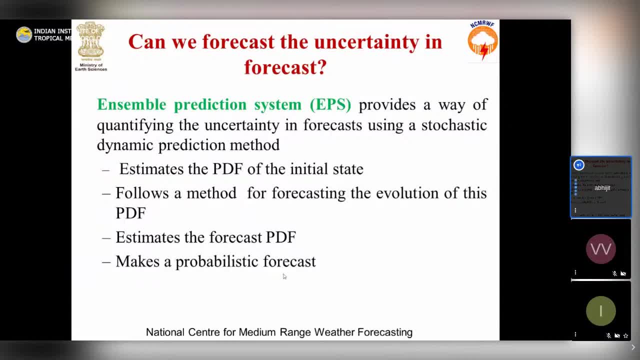 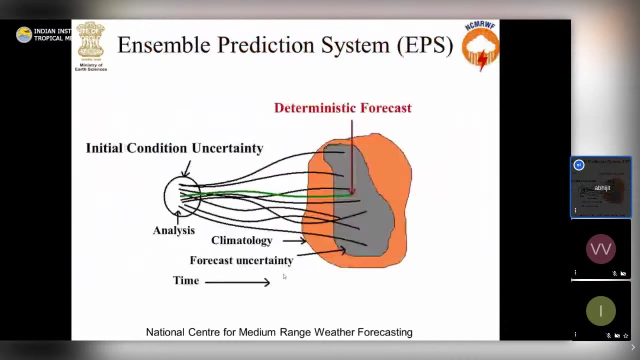 what is the probability density function of the initial state. then, by using dynamical model, we forecast this probability density function and we get the forecast probability density function and from there we issue the probability forecast, probabilistic forecast. so in this method, what we do. so this is just giving a simplified 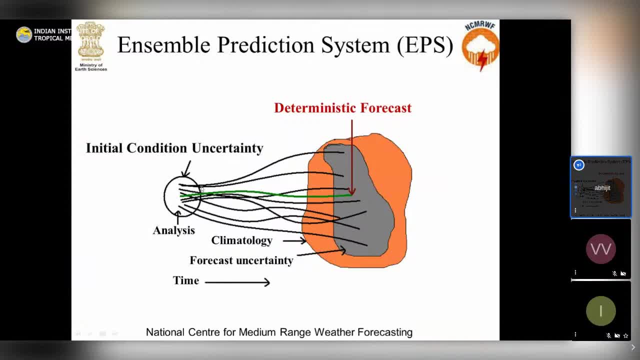 explanation how we create ensemble prediction system. so this small circle, it indicates the initial condition: uncertainty. so from there, so multiple models, we are giving us the forecast. all these models, they are very similar to each other, but they are not identical to each other. so all these model physics, parameterization schemes, we just model physics. 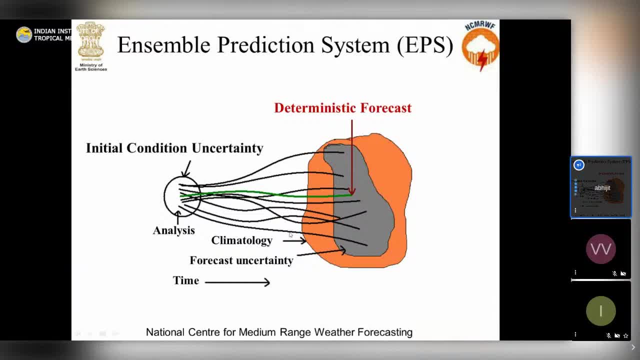 parameterization schemes. we pattern little bit so that the model physics is little bit different from each other, and this initial conditions also. we pattern so that initial conditions are little bit different from each other to cover the whole uncertainty range in the initial condition. so that means to cover 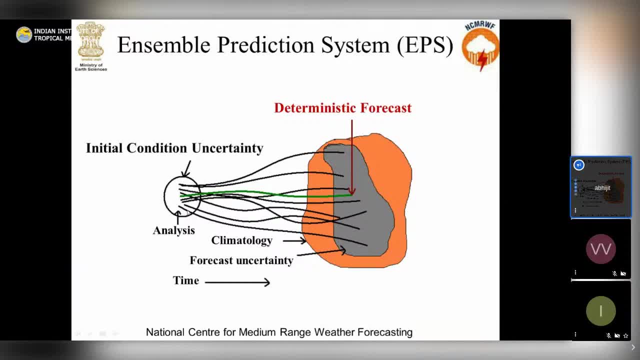 the whole probability density function of the initial condition and from there, whatever the forecast we get, so that we get the forecast. so this black part, this gray part, it is giving this forecast uncertainty. so we can see this initial condition uncertainty. it has grown so forecast uncertainty is larger than the. 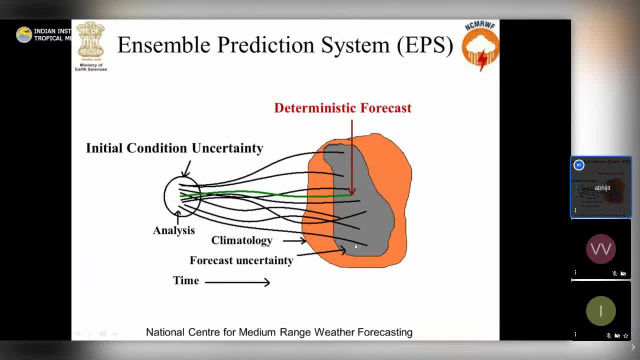 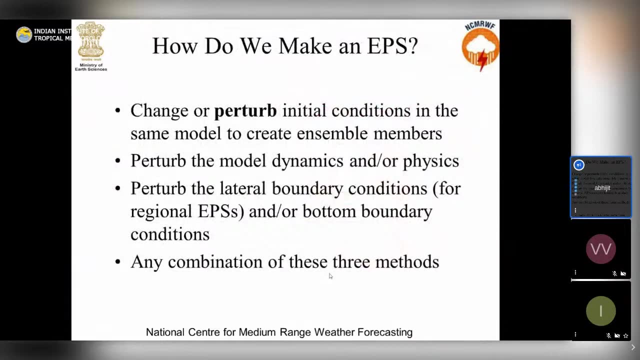 initial condition: uncertainty. now from the number of the members we can calculate that what will be the probability of the forecast. how can we make this ensemble prediction system? we can change these or part of these initial conditions in the same model to create ensemble members we can part of. 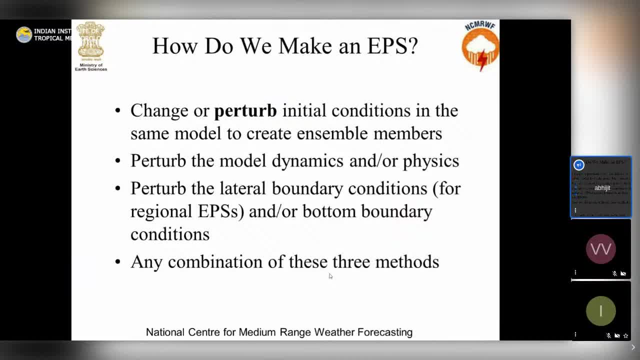 the model dynamics or the model parameterization scheme or physical processes. we can part of the lateral boundary conditions or the lower boundary conditions and any combination of these three methods. so by using these methods we can produce multiple forecasts. so that means we can produce multiple scenarios and from these multiple scenarios we can express these: 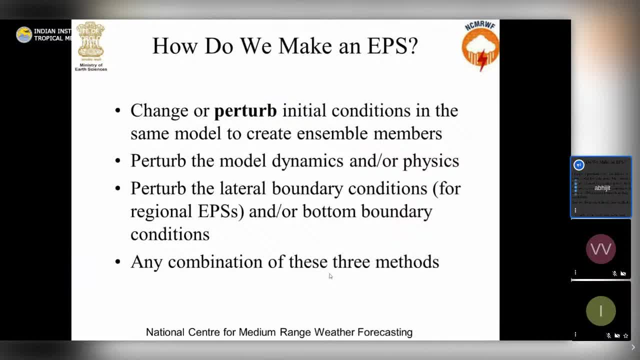 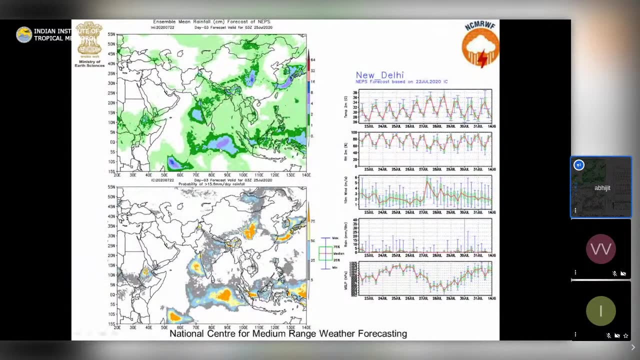 uncertainty in the forecast in terms of the probability of the forecast and the, in terms of either spread or disagreement between the members, or in terms of probability of the forecast, like this is giving this mean forecast, mean precipitation forecast, so which is filtering out all these less probable? 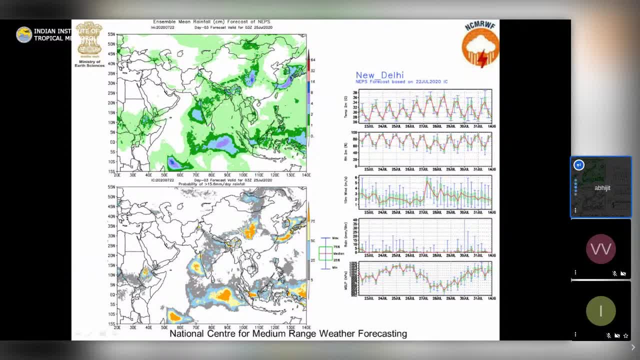 forecast and which is giving the mean of the all the members. this is giving us the probability forecast. so it is telling that what is the probability that rainfall will be greater than 15.6 millimeter per day on 25th July? so if we have 20 members in the ensemble, if 15 members out of these 20, 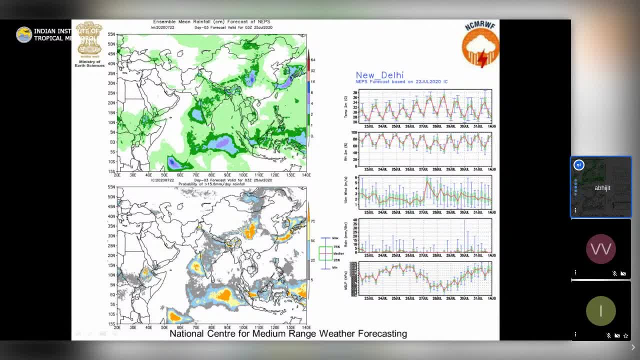 so they can. they forecast that greater than 15.6 millimeter of part dale in fall. so then will tell that there is 75% probability that the rainfall of rainfall will be greater than 15.6 millimeter per day. so this color, which is giving us the 75 percent beta-10, 75% for unity, this blue, 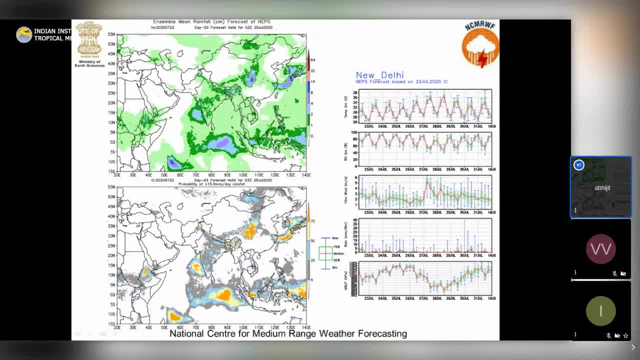 color it is giving that, this blue color, it is giving us the probability. it is is greater than 25 percent, but less than 50 percent. So if we have 20 ensemble members, so it is giving more than 5 members, so that between 5 to 10 members are predicting the 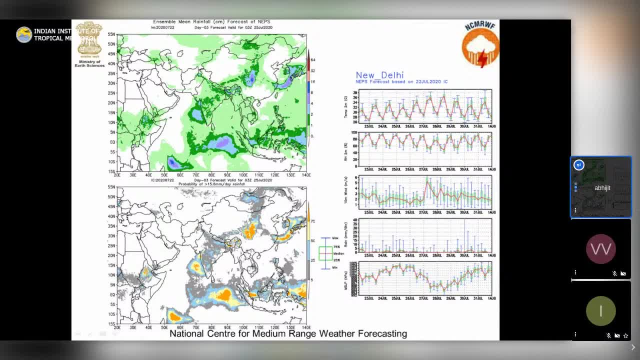 rainfall greater than 15.6 millimeter within this in this region On the right side. it is giving us that we call it is EPS gram or ensemble meteogram. So, unlike meteogram, it is giving us that how many members are giving us a particular? 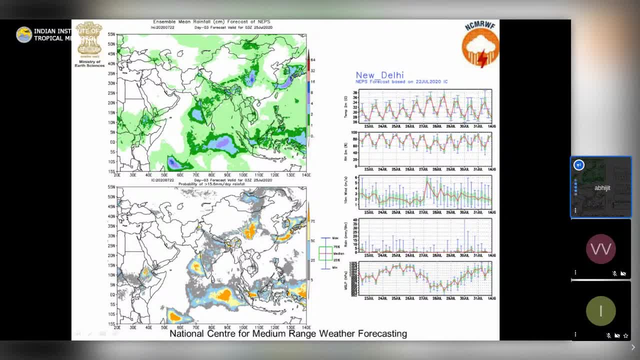 forecast like this is rainfall forecast. So this top of this green box it is giving the 75 percentile. The bottom of this green box it is giving 25 percentile and the middle, the red line, it is giving us the median. so So if we see this middle, this red line, at this time it is giving us- suppose it is- 4 millimeter. 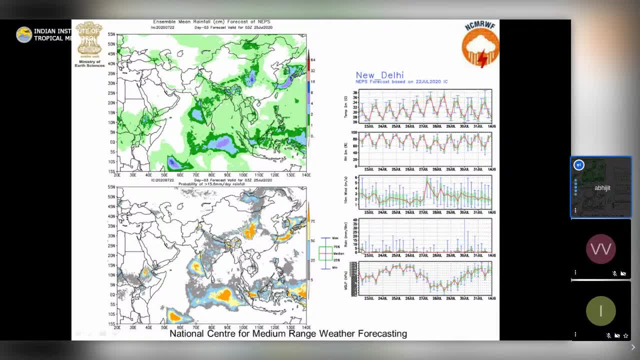 members are giving the forecast the less than 4 centimeter, 4 millimeter, and rest of the members are giving the forecast above 4 millimeter per 6 hour rainfall. So in this way we express that forecast uncertainty in terms of probability. So 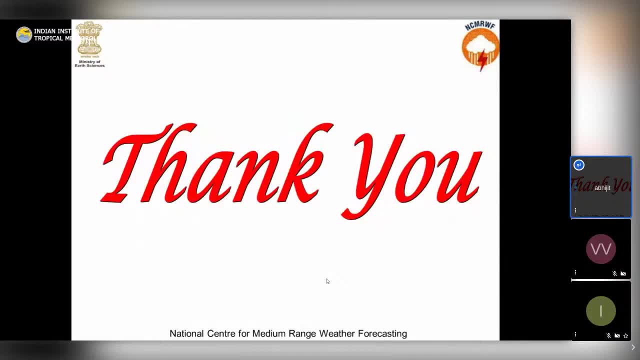 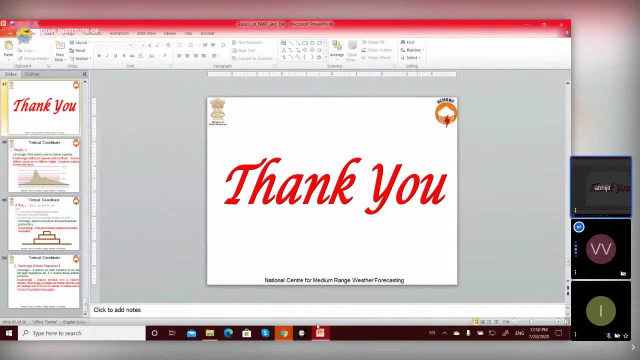 that's all from today's webinar. Thank you all. Thank you, Dr Abhijit Sarkar. It was a very interesting and basic talk on NWPN data assimilation. So there are several questions it gathered. So can you please stop the screen sharing and come? 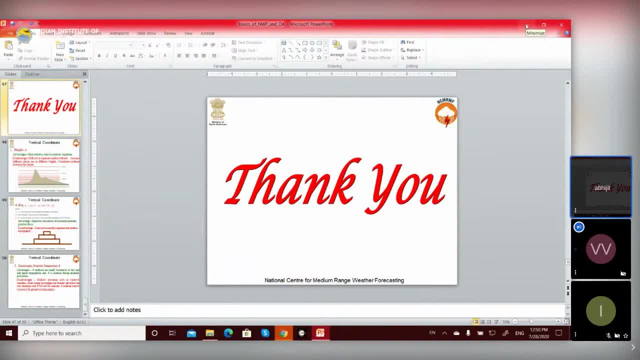 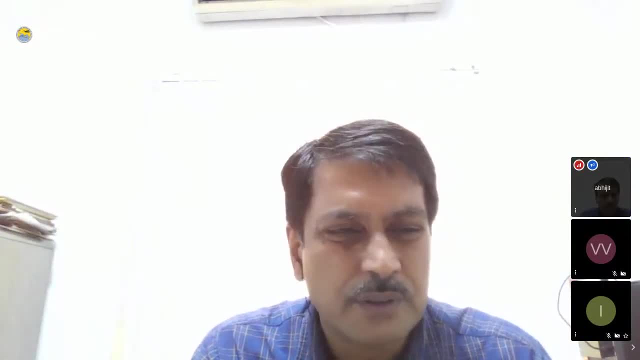 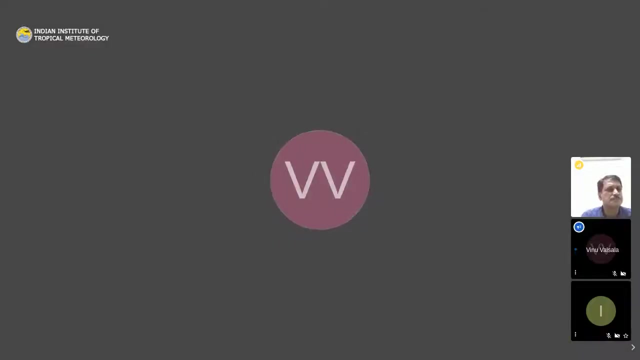 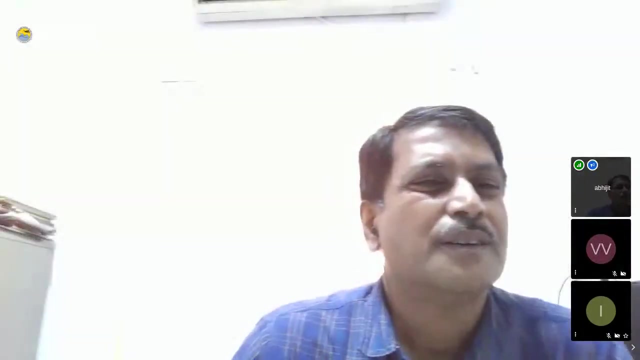 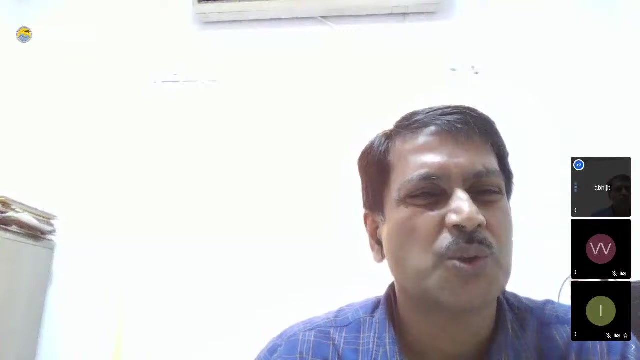 out. I have placed the question in the chat window. Have you seen the questions? Just open the chat window. Yeah, chat window. There are questions. Yeah, first question is that: what are the advantages and disadvantages of standalone atmosphere ocean model and a coupled model? So advantages. 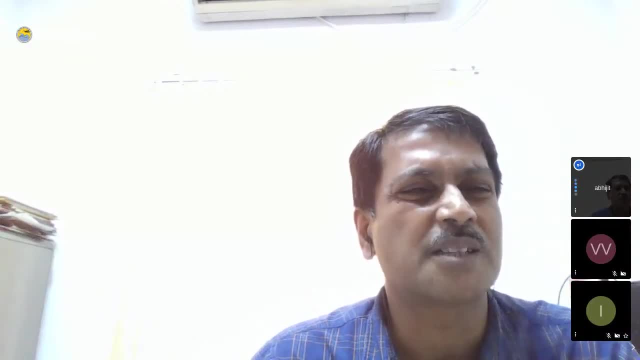 and if it is short term atmospheric forecast, so then ocean condition does not change that much. So if we take these ocean models of, if we include the ocean model also, So then it will be very much expensive. So within a short forecast time the ocean surface or ocean condition does not change much. So 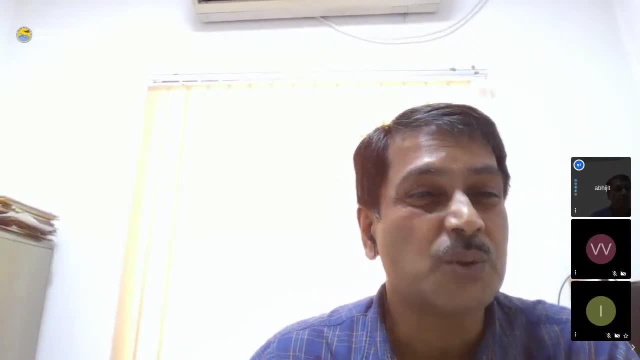 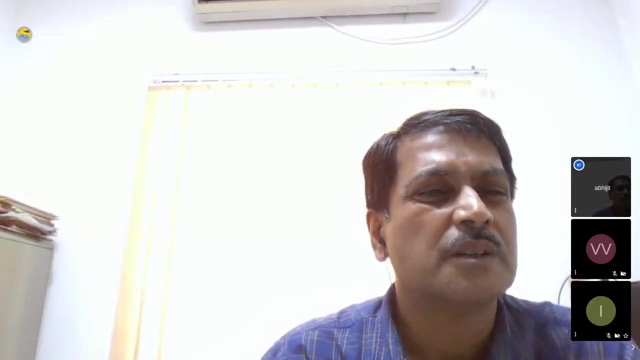 if we, if we can include these ocean model, so that is good. But it we have to see what are the means, what is our resources. so depending on that we can include this atmosphere and ocean coupled model. and but if, if we any can include, it is always good. and then second is kindly explain the ncmr dolly. 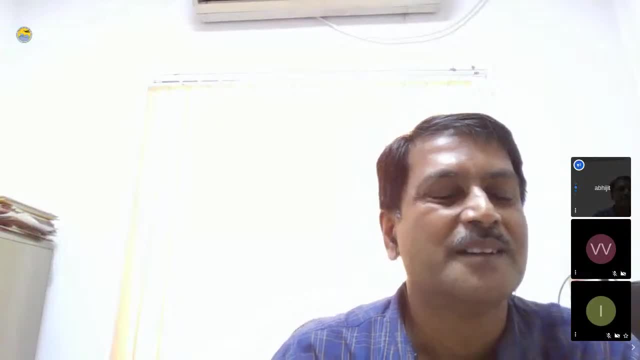 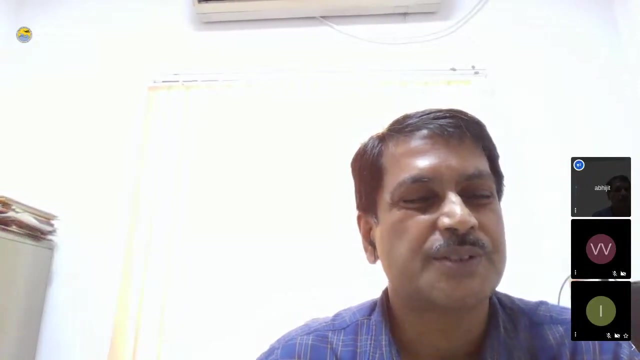 pension will be in simple prediction system, ncmr dolly pencil prediction system. so that is based on these unified model developed at mid-office in K, and this ensemble prediction system has total 23 ensemble members. I have talked about what are. what are then? so what do you mean by ensemble members? that is, 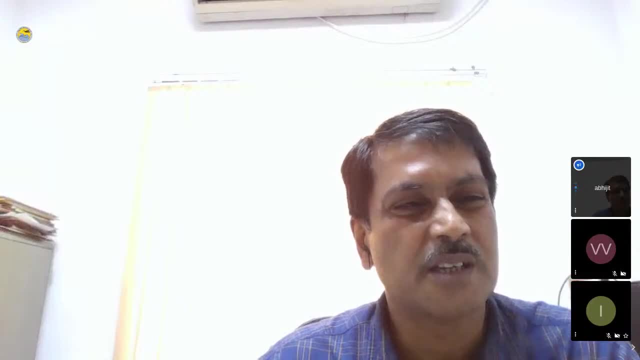 11 ensemble members. it start from 0 UTC of the current day and then 11 ensemble members. it start from previous day, 12 UTC. so do we create this: 22 members, 22 part of members and one deterministic focus that we use, that control focus. so 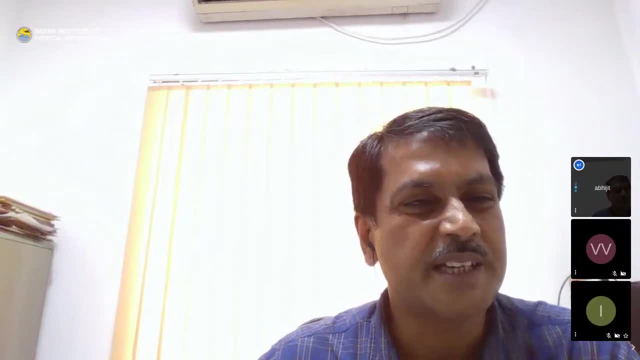 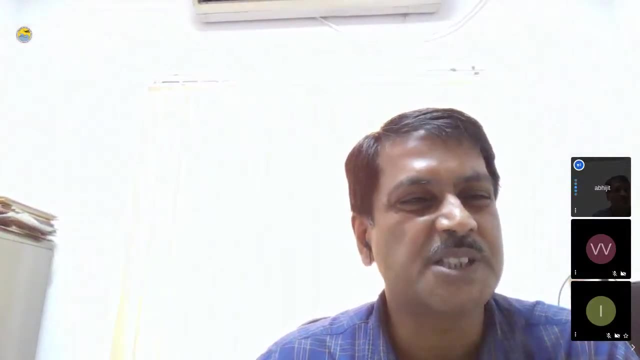 there are total 23 ensemble members. we create the pattern vision by the method of ensemble transform, column and filter, when its initial condition pattern and the physics perturbations we generate using the stochastic kinetic energy back scattering method and which commit in combination with the random parameterization scheme. and second is: what is the significance of staggered? 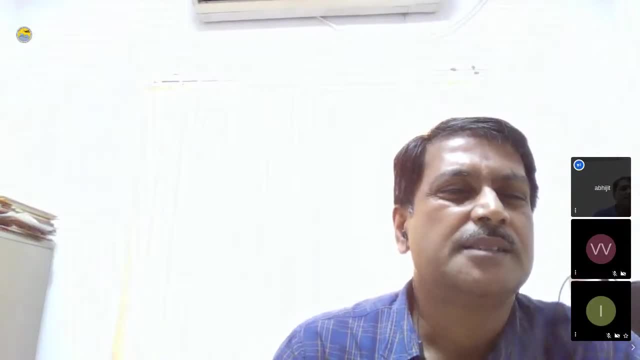 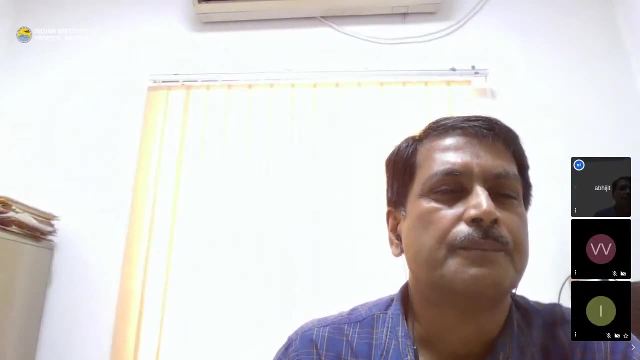 grid. actually the staggered grid is staggered grid is used to replicate the dispersive property of the actual waves which are which are present in the atmosphere. so it has been seen that C- staggered grid and E staggered grid. they can properly replicate the dispersion property of the waves that are actually prevalent in the atmosphere. 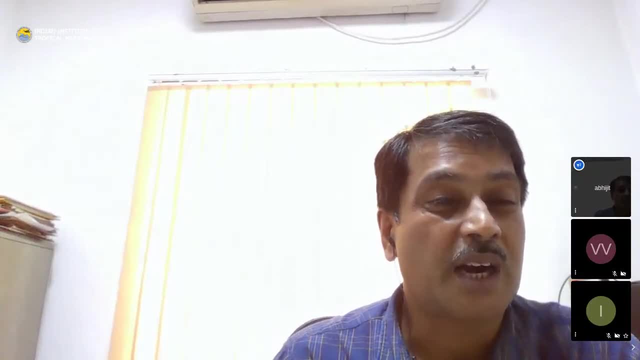 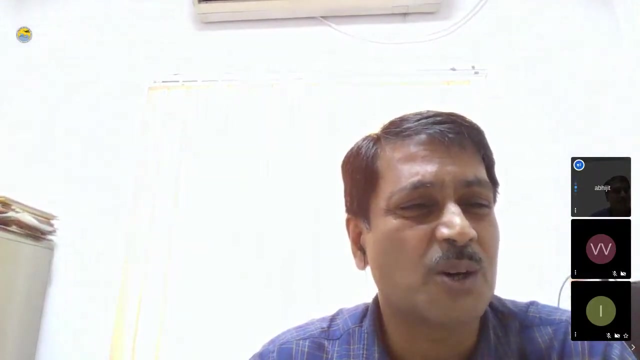 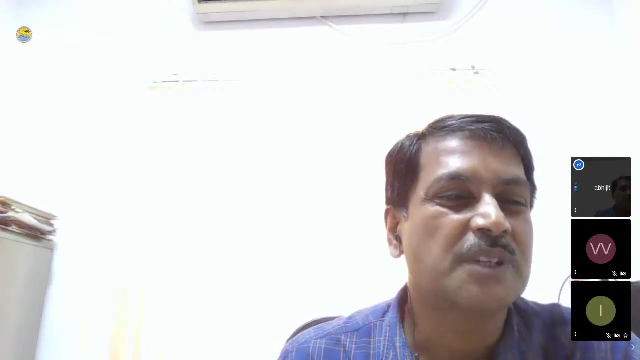 so most of the models they use Arakawa C grid and Arakawa E grid, but Arakawa C grid is considered better. and fourth question is: what are the advantages and disadvantages of WRF models over coupled models? couple model: of course it will be expensive. WRF- 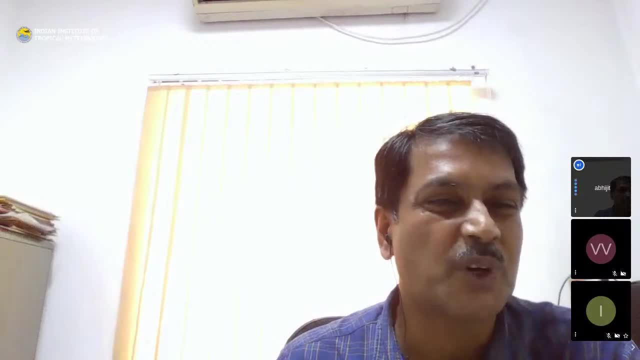 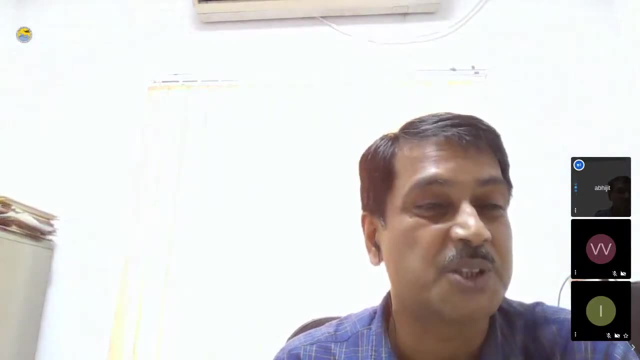 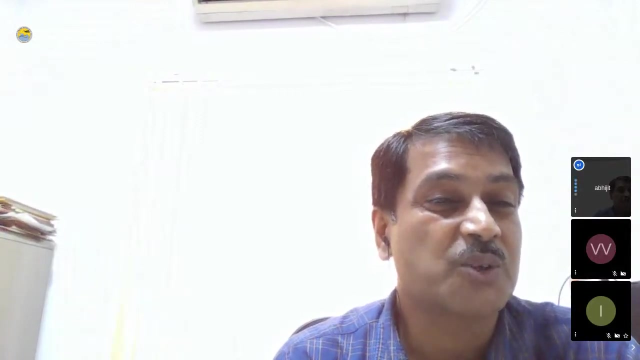 model is a atmospheric model, it is a Grid Point model. so whatever the advantages and disadvantages associated with the grid point model, that will be there with the WRF model. but we are not considering the variability of the ocean, we are not including in this forecast, so there will be disadvantages means if we want to give a long range forecast. 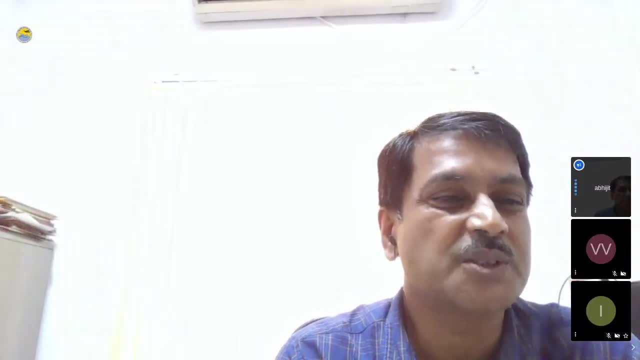 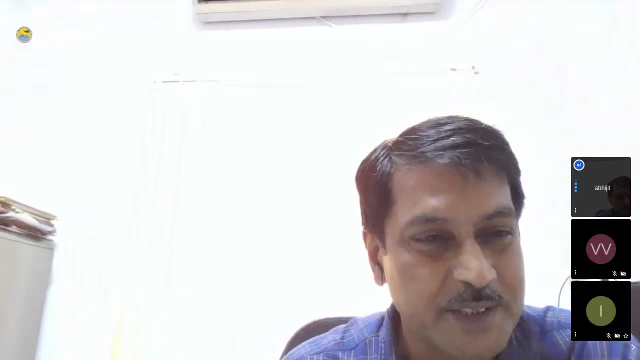 with the help of only atmospheric WRF model, so then the forecast will be erroneous. What are the challenges for numerical weather prediction in tropical region and its accuracy compared to mid-latitude region? In mid-latitude region, the weather systems are generally advective and models are very 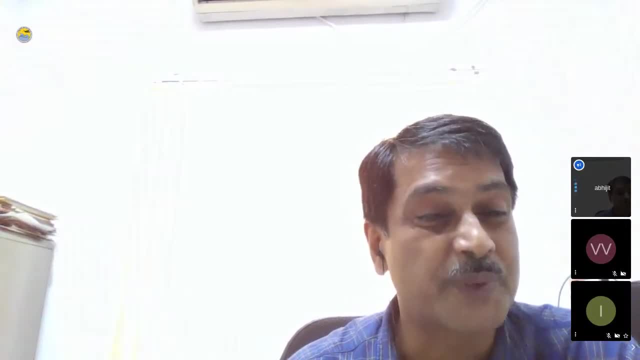 well to predict, very skillful to predict those adverse weather conditions, Advective weather systems, whereas this tropical atmosphere, it is this small-scale convective phenomena dominate. so it is difficult for these numerical weather prediction models to predict in this tropical region.